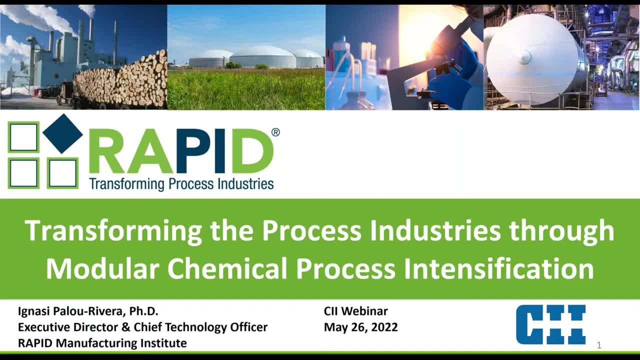 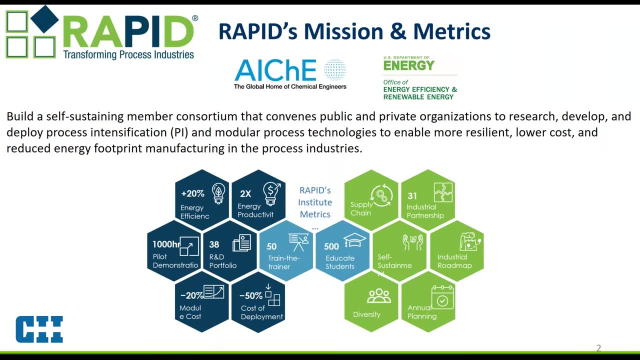 And I'll present who RAPID is. And, as you see here, you know, RAPID is really a collaboration, what we call a public-private partnership, between the American Institute of Chemical Engineers and the Advanced Manufacturing Office of the Department of Energy. Okay, So the 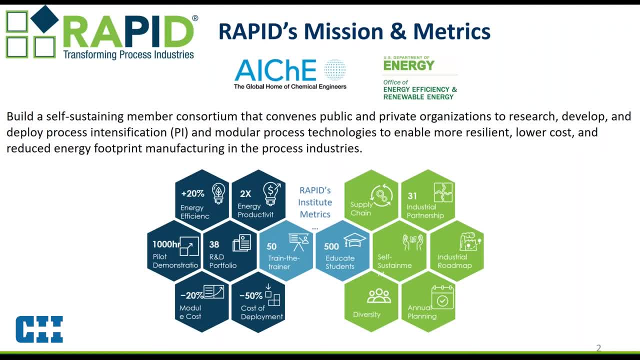 Advanced Manufacturing Office is part of the Office of Energy Efficiency and Renewable Energy of the DOE And AICH, the American Institute of Chemical Engineers, who I am both a member and an employee of. So RAPID is a part of AICH. that managed manages a grant, an agreement, a cooperative. 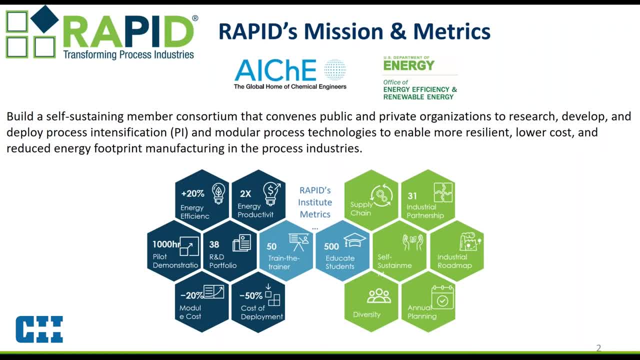 agreement from the DOE to do work And as part of that, we are in charge of building and managing a self-sustaining consortium to bring these public and private organizations to work in the topic of process intensification and modular process technologies to enable 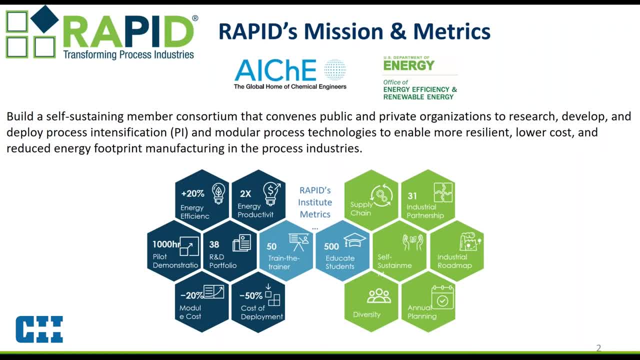 as it says there, a more resilient, lower cost and reduced energy footprint for manufacturing in the process industries. So what you see, there are those hexagons as some of the metrics that we were given by the DOE, that we've been working towards for the last five plus years. 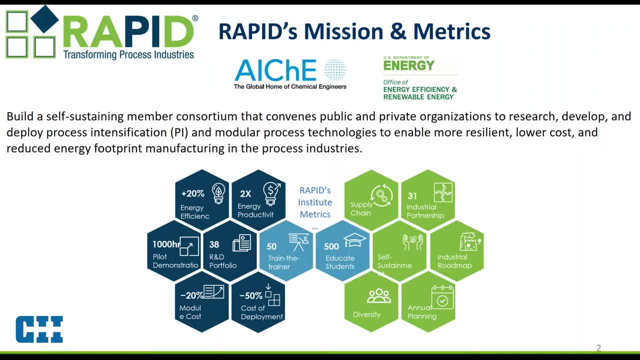 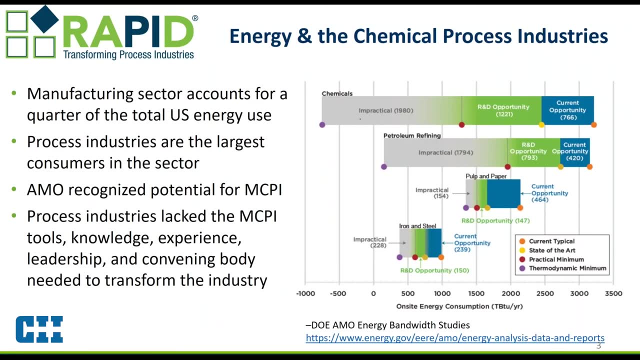 in terms of increasing energy efficiency and energy productivity, reducing module costs and the like. So why was a DOE and why were? was AICH interested in working in this area? A bit of a background and I'll try to go through this a bit fast. I think it's relatively easy to. 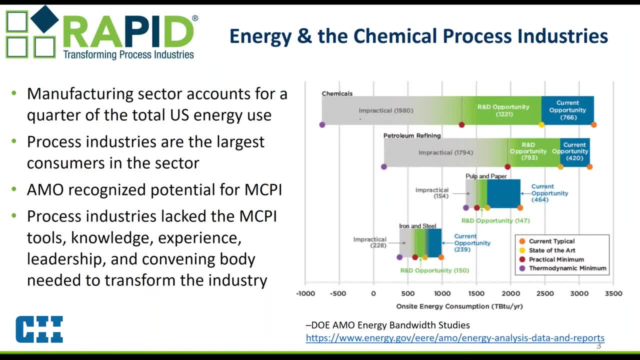 understand for those of us that have been in the process industries for a while to understand that the manufacturing sector, and within it the process industries, are a very large user of energy. in this case in the US right so manufacturing center about a quarter of total US energy use. 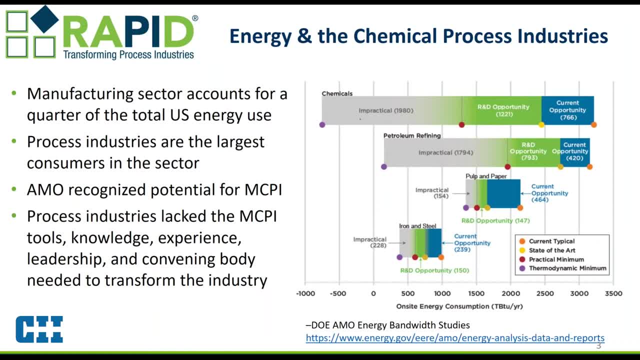 with the process industries being the largest specific sector in manufacturing. so AMO, the DOE, recognized the potential for MCPI, these modular chemical process intensification that I will define in a minute, and set up a rapid or the initiative. that became rapid as an institute and realized that the process industries- there was really no organization, that a combined tools. 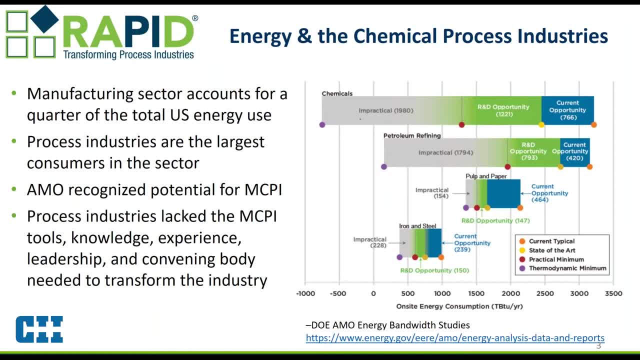 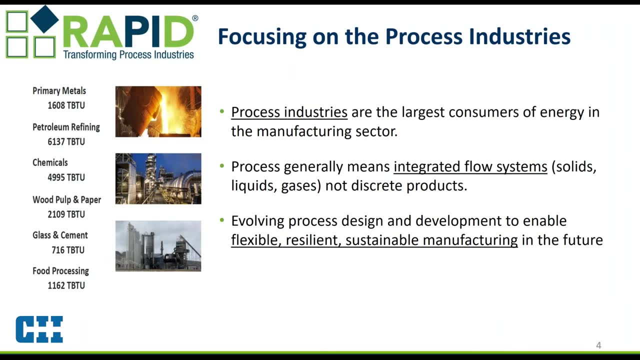 knowledge, experience, leadership and act as a convening body. so rapid became that competing body and was able to do that. We have been in operation since 2017 doing just that work. Also, when we talk about the process industries, I wanted to emphasize that we're talking. 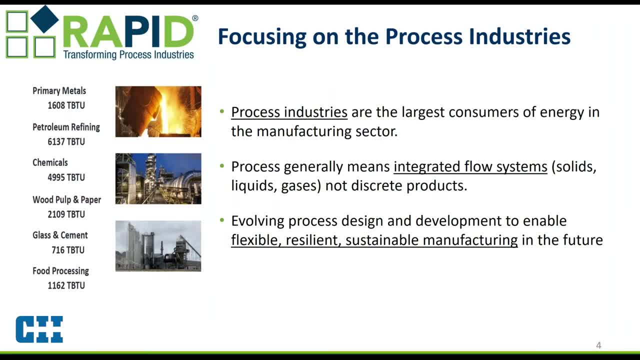 a bit broader than the strict kind of chemical and refining industry. we are talking about industries incorporating things like metals, pulp and paper, wood, construction materials, food, glass and cement, food processing in general. everything that in the process industries are doing is based on integrated flow systems as opposed to discrete. 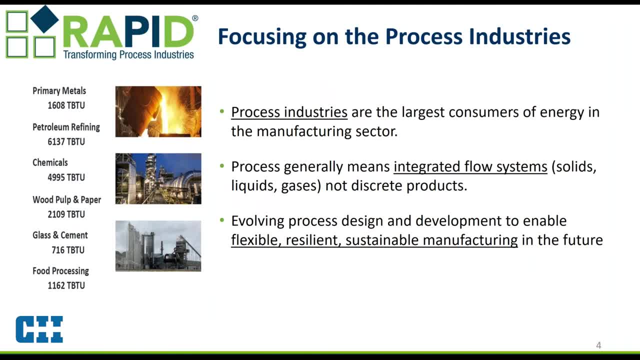 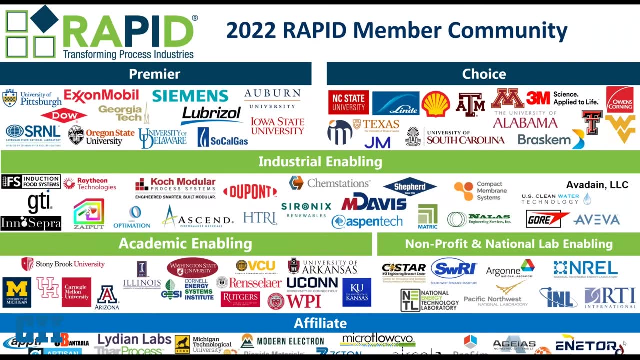 products. So very critical that we are looking at these wider industry manufacturing sector. So rapid is a membership organization similar, or, you know, parallel to what CII is. in that sense our membership is made of organizations, not of individuals. Here's a snapshot of our current, or at least current as of a few weeks ago. it changes a bit. 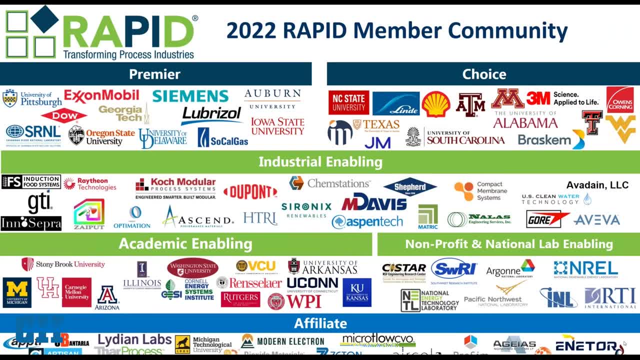 as you can imagine, of the 2022 rapid member, a community with the different levels of membership. I wanted to bring this slide because I am sure that there is many of you here who are attending us involved in CIson. there are actually in one of these rapid membership organizations. we know that. 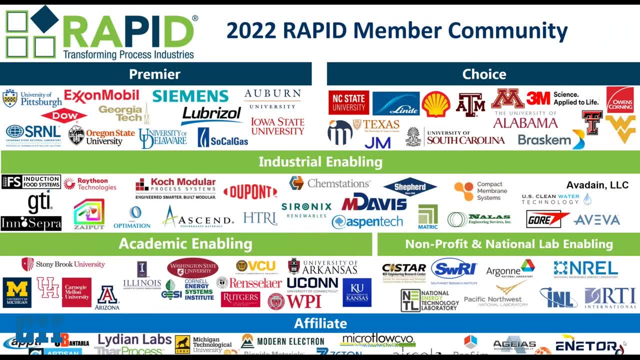 there is many companies that are both members of CII and members of rapid. many times the folks within those companies that are engaged in the different consortia are quite different and there is sometimes not a knowledge or not an understanding that there is so much common membership, as you see here- rapid- 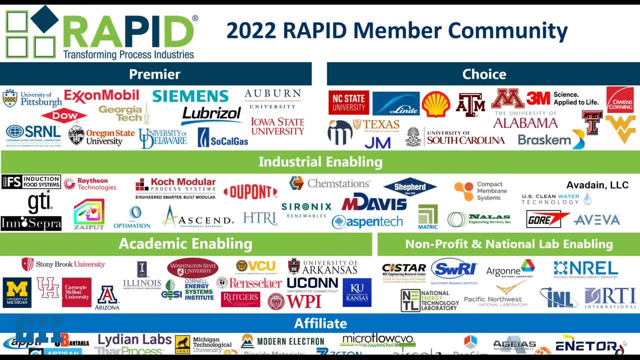 has different types of members. we have industrial members at different levels and you know large companies, medium companies, small companies. but we as well have academic and nonprofit and national lab members. as you see here, affiliate membership is those kind of a being engaged but not quite as integrated in. 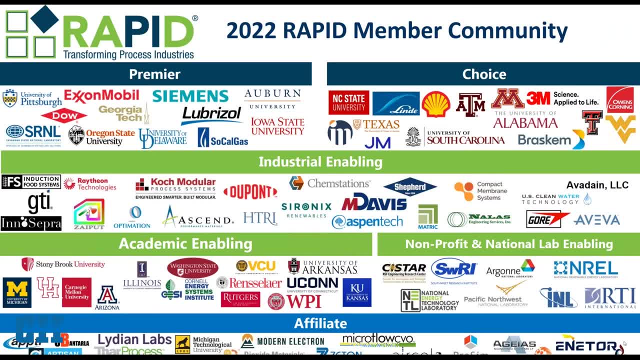 rapid. so obviously any of you in these companies or other companies that have an interest in what rapid is and what rapid does, feel free to reach out. if you're already a member of rapid but you don't know who to contact, our website lists the member representative. 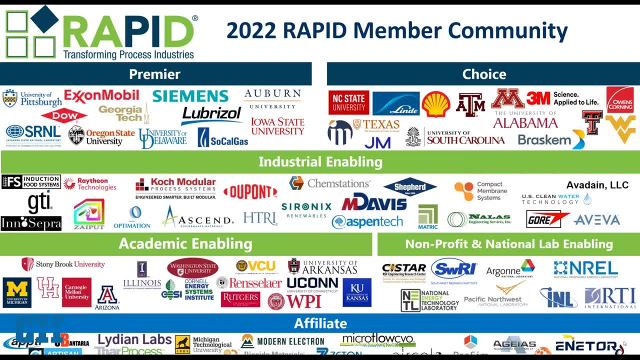 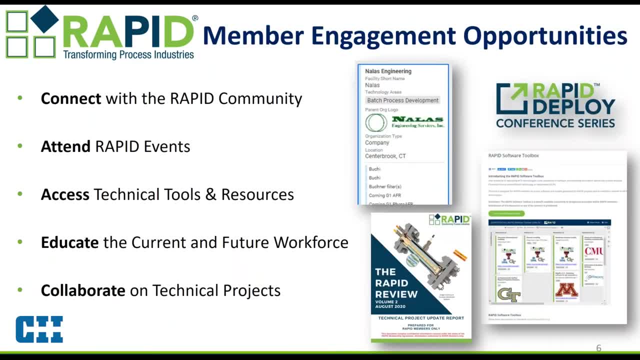 for that specific organization or we can help you find out so that you can work with us a bit more. you know some of the some of the regular member engagement opportunities I have to put in a plug for rapid membership, even though this is not really the focus of the talk. you know we 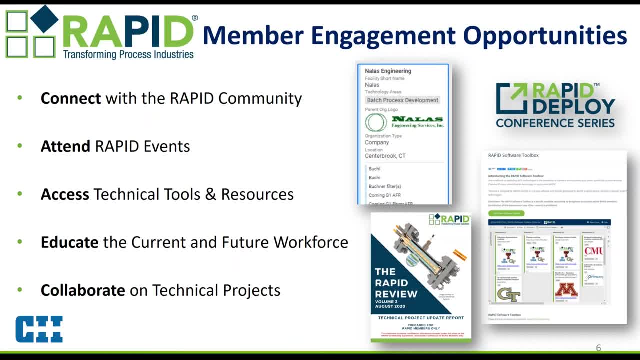 are a community convener. we have our own a series of events. we just started rapid deploy conference series, which is kind of a hybrid between a workshop and in a conference. very interesting concept. a number of technical tools and resources, rapid test network software toolbox that we share with the members. very strong a. 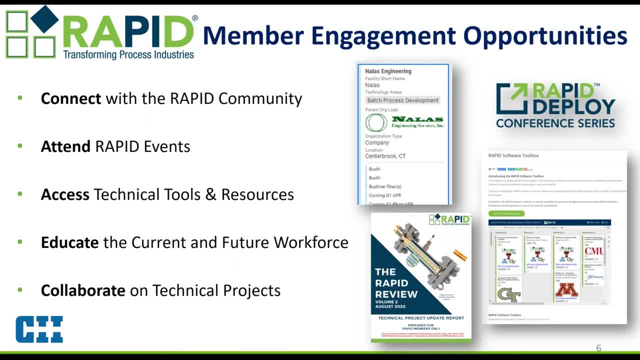 very highly praised educational and workforce development activities, some presential, some virtual online, and then collaboration work on technical projects, which is how the collaboration between rapid and and CI was established and performed, and I'll be and to detail a little bit, so I wanted to spend a couple 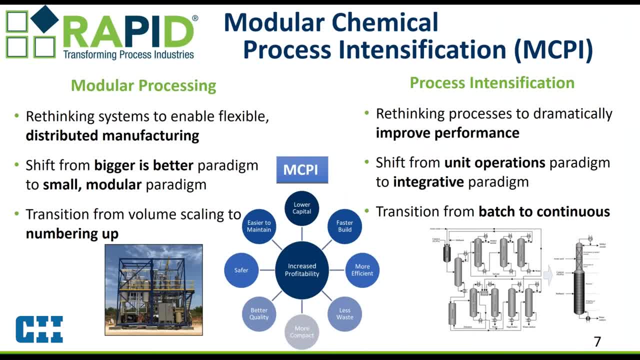 of minutes here defining these idea of modular chemical process intensification, what I sometimes call our sandbox- so these is gonna be original area in which rapid was established to work in, and CPI for short. this is the combination of two concepts that have been and are familiar to a lot of chemical engineers in 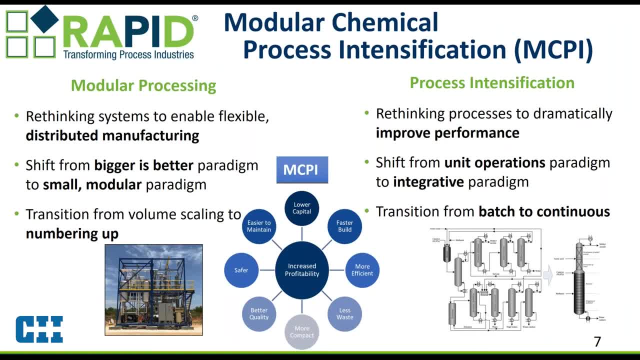 the module. I would say to others as well. but I wanted to to kind of bring up up the two concepts and then how we connect them and how we see extra value when that connection is done. So I'll start with process intensification on your right side of the slide there. 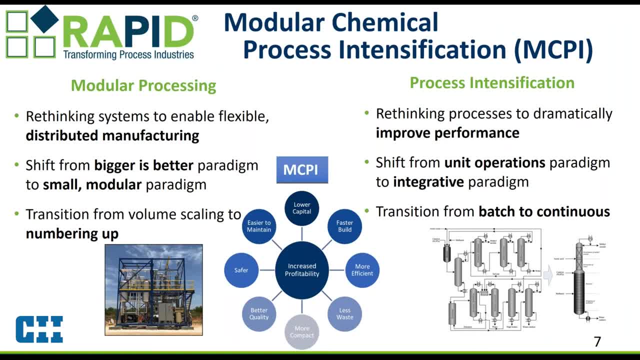 So process intensification is a concept, an idea in the chemical engineering world has been around for a while, is hard to define, is really one of those difficult to define ideas, but it has a fairly well-distinguished personality From the rapid side. we look at it as a way to rethink process and process development. 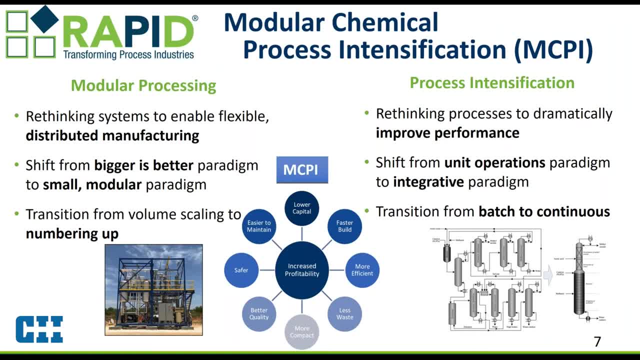 process design to dramatically improve performance, This idea of dramatically make huge gains in energy and capital efficiency, for example. Important point: The shift from Separate unit operations, the paradigm of kind of stringing unit operations to make a process, to a more integrative definition or design of processes in which we combine 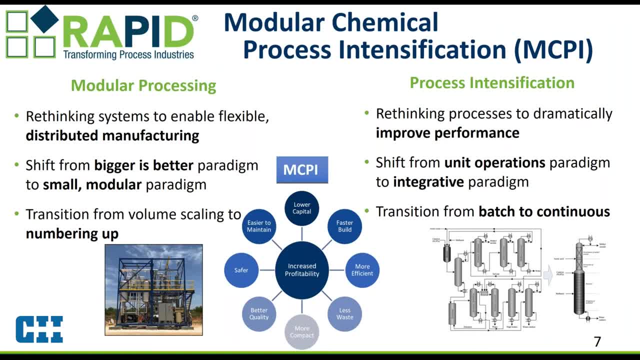 the phenomena that normally occur in separate unit operations, within these integrated, these intensified operations. Very basic example would be the transition from a batch process Process to continuous process. In one of the case examples that our collaboration address was very much in that area. 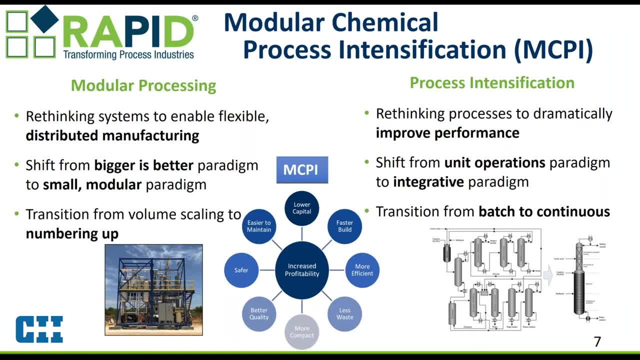 The cartoon you see there at the bottom is one of the classic examples of process intensification. That's the intensified methyl acetate process that Eastman Chemical created. or did You see there the original process, Many different units, Many connections- that was intensified into a single unit, into a single single reactive. 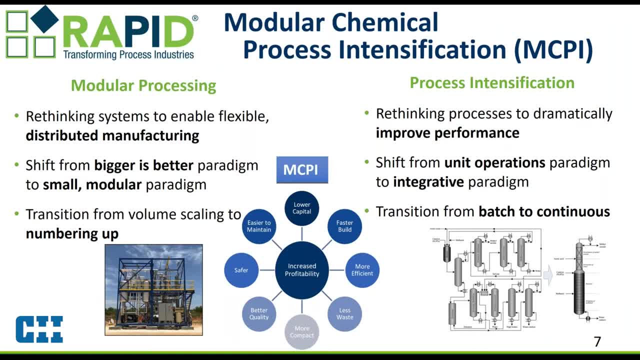 distillation unit. So what you see is one unit instead of many, a more complex, a more integrated unit, but a much more efficient and energy capital efficient. So this is what process intensification is, or how we address it: Modular processing. 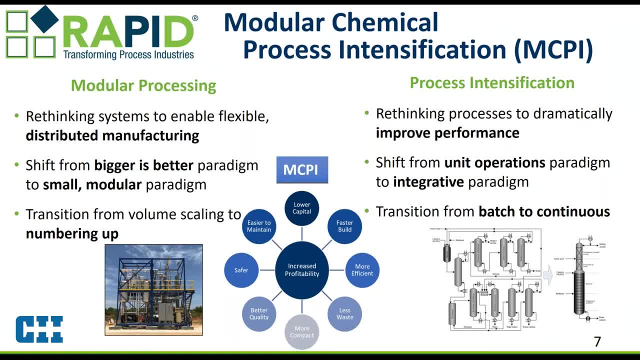 Also a number of different concepts that folks have done in the module processing world. The way we look at it from the rapid perspective is this idea of rethinking systems to enable flexible and distributed manufacturing. So we are looking at complete modular systems, not at not the Lego approach of many pieces. 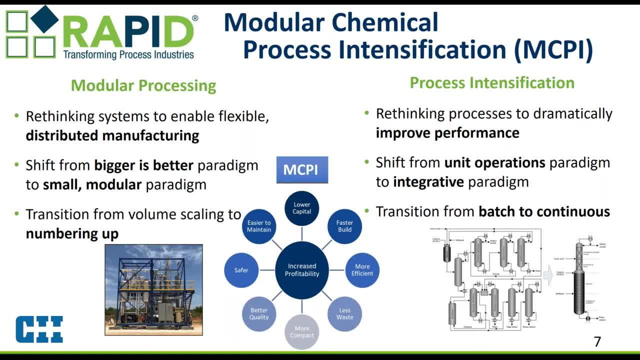 into many modular pieces to make a larger process, Okay, But more of a smaller repeatable processes, so that we can go from a paradigm of a bigger, is better. So the scale up traditional approach and in the process industries and chemical engineering to these smaller modular paradigm in which the scale is not done in volume but in numbering. 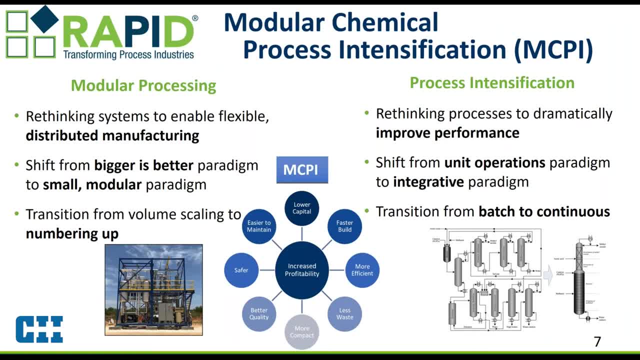 up. So we go from a, you know, larger units in order to take care of the process, to a larger unit In order to take care of its economies of scale, into numbering up in standardized units of modules in which there is no need to re-engineer each cases. 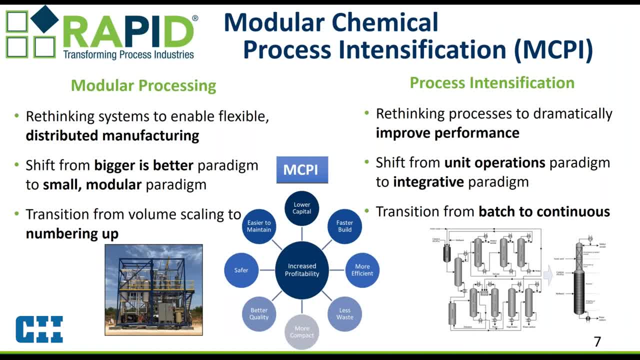 So when you combine these two ideas- process intensification, modularization- into the NCPI, you can, and we have examples And that's what we want to talk to you about: The children. The kids show a large increase in profitability from concepts such as faster wheel increase. 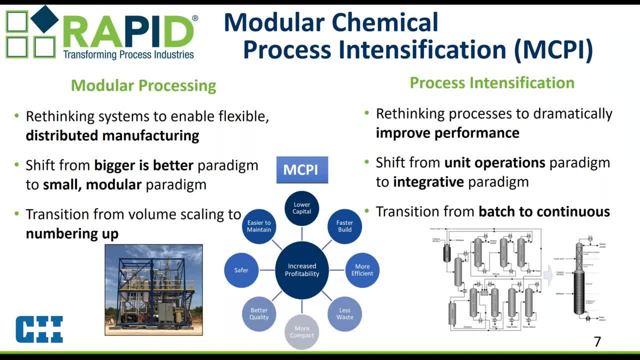 efficiency, compactness, increase in quality, safety, lower maintenance, lower capital costs, And we'll bring up some of the examples that that give rise to these potential increase profitability In rapid. We've been organized for a while now into a number. 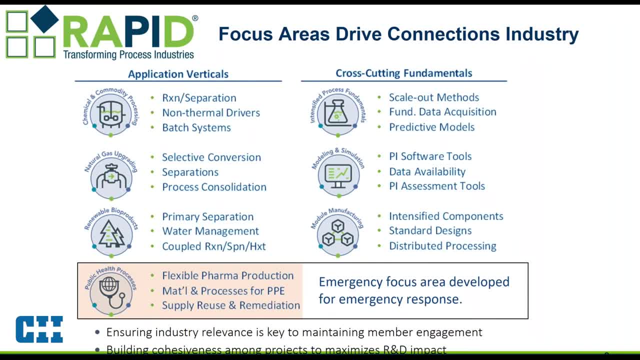 Of focus areas, some looking at application verticals in the industry, some looking at cross-cutting fundamentals- And I wanted to bring these organization because the way that we came out to work with CI and the project that I will present just in a minute I came from very much one of these. 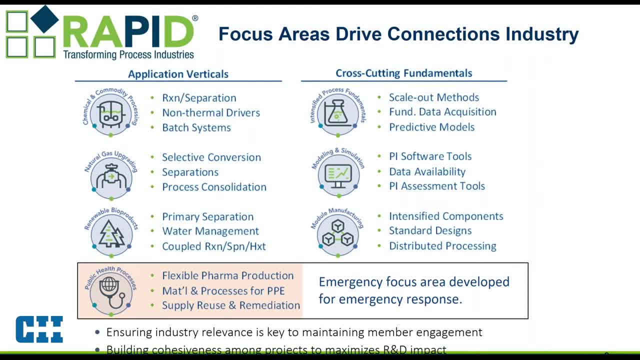 focus areas is is is focus area, the six focus area that you see here in rapid. that's kind of focus area 10. Which is module manufacturing, In which these idea that, in order to take advantage of modular production, we need to. 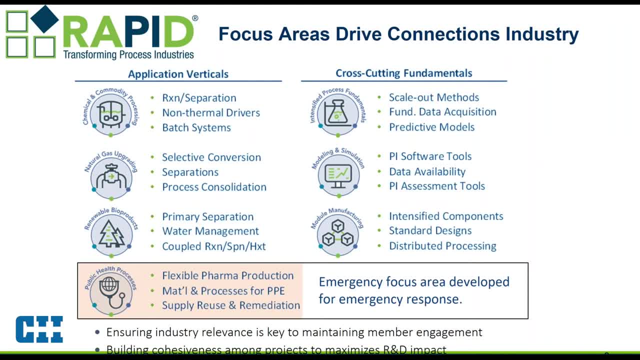 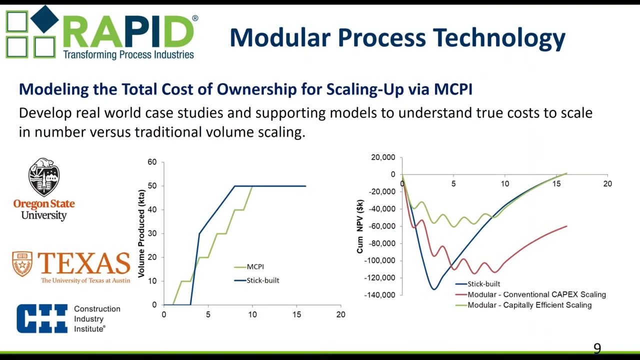 better understand the costs of fabricating, designing and then the the repeated fabrication of modules, this numbering up. So, within this module manufacturing focus area, We started a project, Which is What I will present here, Looking at understanding the cost of really scanning, scaling up via MCPI, via a numbering. 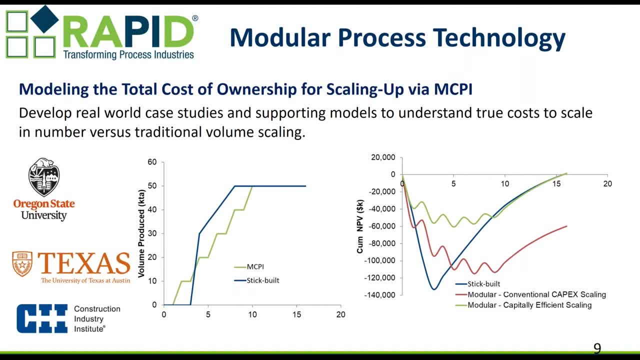 up of modular intensified units. Okay So, modular manufacturing focus area sponsored these project and the project was performed as a collaboration between Oregon state university and their manufacturing engineering folks and the construction industry Institute at university of Texas. So that copy eyes for these project, where Brian Paul from Oregon state and Jim O'Connor 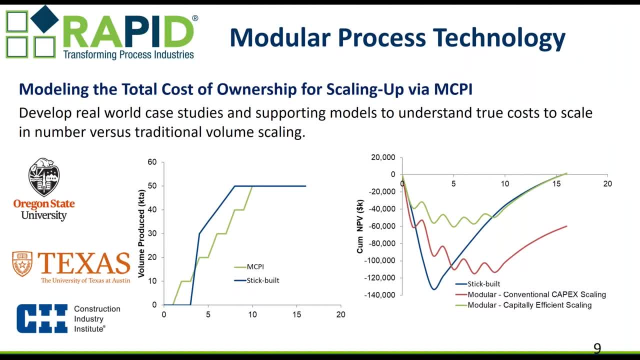 from CII university of Texas and both of them presented at the CI meeting in Orlando last year. So some of you might be familiar with some of the work that they presented when it was a roughly done but not quite Maybe 90% of the work that they presented. 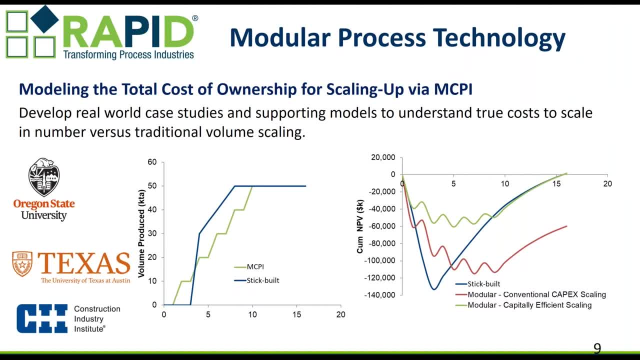 The idea for the project was kind of trying to get some data, in some case studies, to justify these conceptual notional charts that you see here in this slide. So the idea that, for example, the one you see here, module produced versus volume produced. 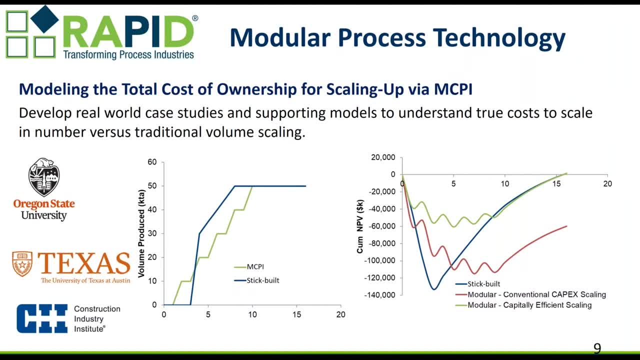 versus number of modules or investment gives you an idea that through MCPI we can scale up production that allows us to go to a large enough production in a more, as I say, scaled up in a more gradual way. In what you see there on the right is that from a, from a, from a net present value. 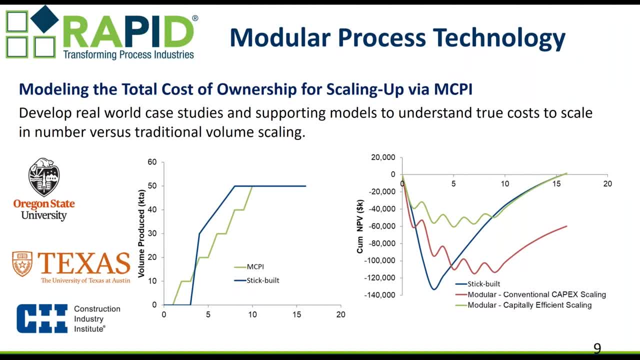 So from an investment, Okay, So from an investment, a return on investment type of approach, a modular way would allow us to get scaling up with reduced initial investment, So a more gradual investment to the larger scale. So to prove these ideas, to prove these concepts, we set up this project and started working. 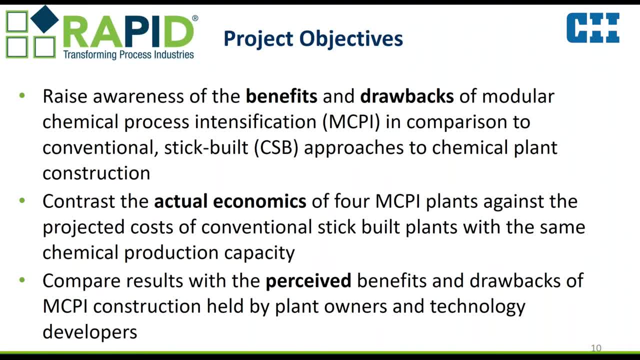 on it. This slide describes the project objectives. So basically raise awareness and really understand the benefits and drawbacks of these two approaches. So the MCPI approach as compared to the conventional or stick built, conventional, stick built, So we use these two acronyms going forward: MCPI, CSB approaches for chemical plant construction. 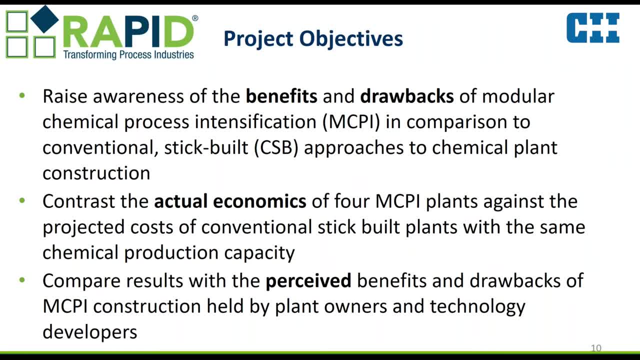 really compare, contrast the actual economics of four. Okay Okay, Okay, Okay Okay. And we model case studies of MCPI versus CSB, with versus conventional stick built and compare the results versus the perception of the benefits and drawbacks. So people have a lot of ideas and a lot of thoughts about in both camps. I would say 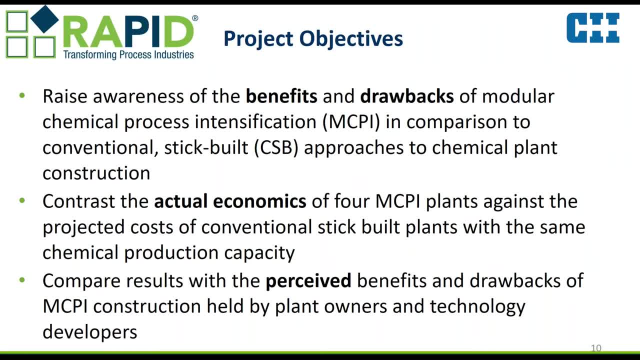 the MCPI and the CSB, but the real amount of data and real case studies based on data is somewhat limited And we really wanted to address that. Let's put some numbers, let's put some studies behind these perceived benefits and drawbacks. 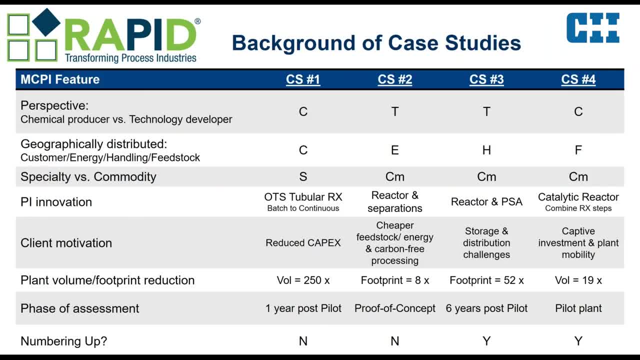 So to do that, the performance that I would say Brian and and Jim with, with the help of the rapid leadership and some of the community, we put up together a slate of four case studies that you see here, trying to cover a number of areas of the process: industries. 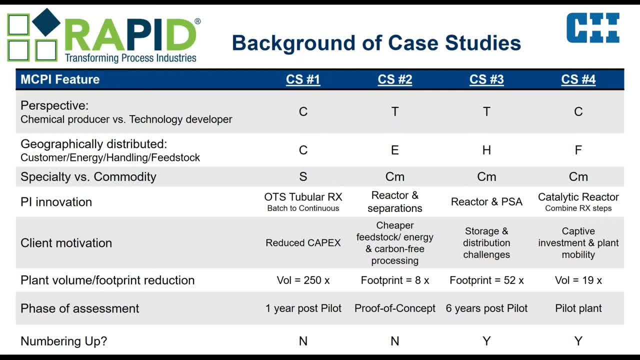 So in this case, case study number one was looking at a batch to continuous transformation, So a large batch processing, as the conventional case, going to a modular continuous approach. So that was intensification, So that was intensification with the motivation of our use capex. 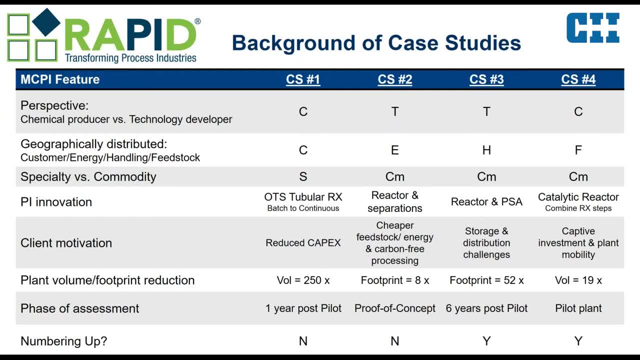 And Jim we'll. we'll talk on that case study in a minute. Case study number two, which was a bit of a tricky one, was looking at more of the idea of a distributed energy resource, And and that one was a bit of a difficult, more difficult one. 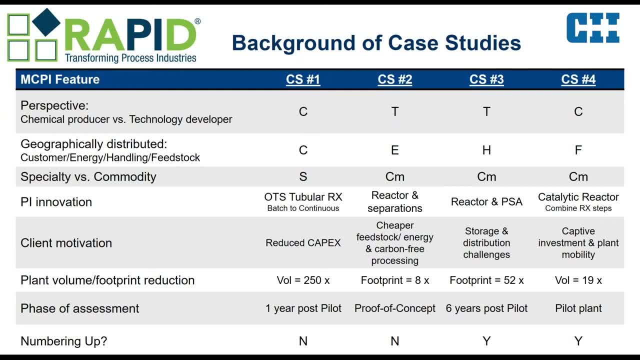 because there was no that the capex data existing for it was at a at a slightly different level, And I'll let Jim and Olivia bring it up that that a bit more detail. Case study number three that I will talk about later was kind of more of a distributed commodity production. 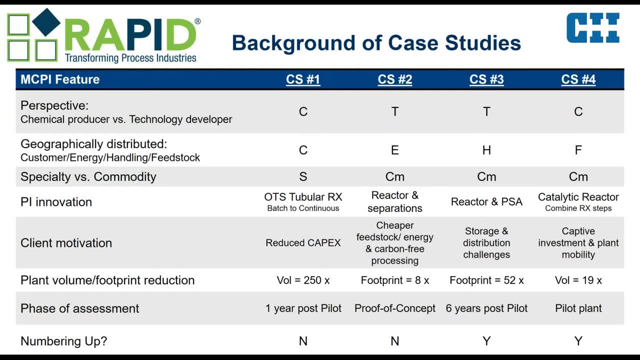 So more of a traditional, large chemical and how to compare the more centralized, scaled up approach that we've all had for years versus these modular, distributed and that idea of numbering up. And then we had the fourth one, which is a distributed or a catalytic, a natural gas processing, trying to address 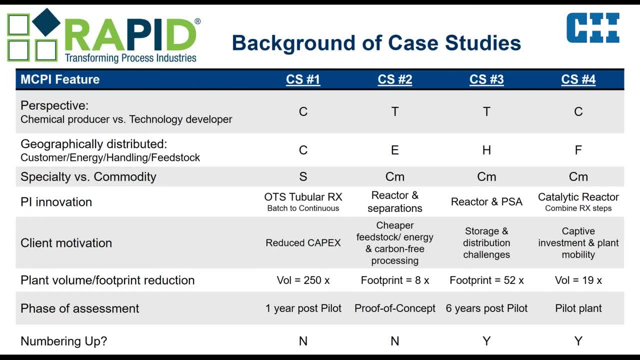 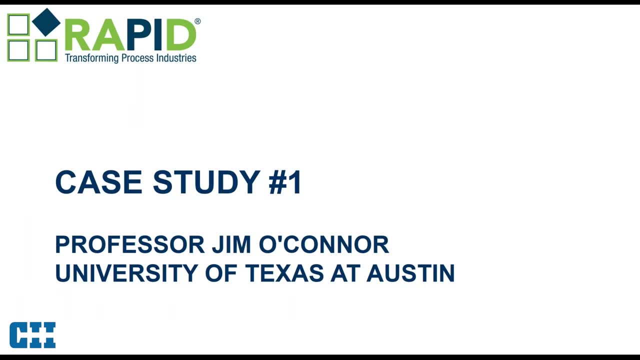 processing distributed non-conventional natural gas. So different cases, different approaches. We'll get into detail in a couple of them, particularly one and three. So I'm going to pass The, the, the, the voice to to to Jim O'Connor at University of Texas. 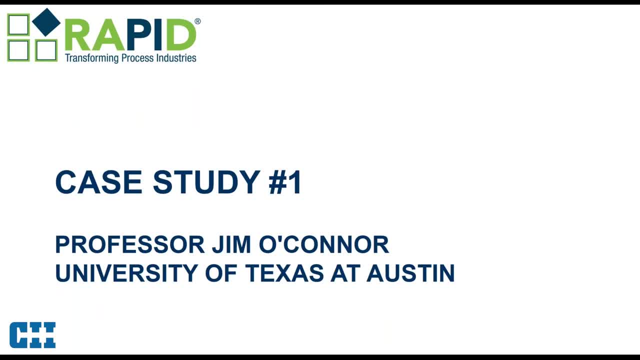 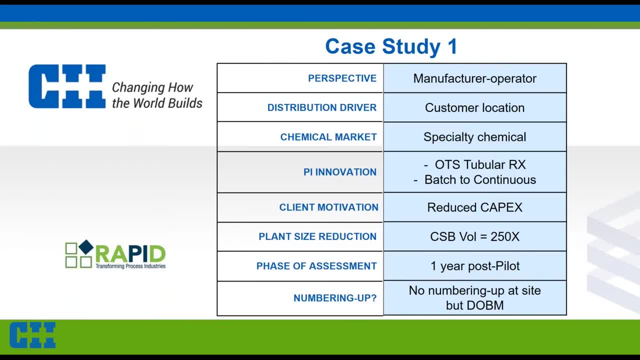 to present case study number one. So, Jim, thank you, Ignacy. Thank you very much. Yes, this is Jim O'Connor from the University of Texas at Austin And, as Ignacy mentioned, I was one of the one of the. 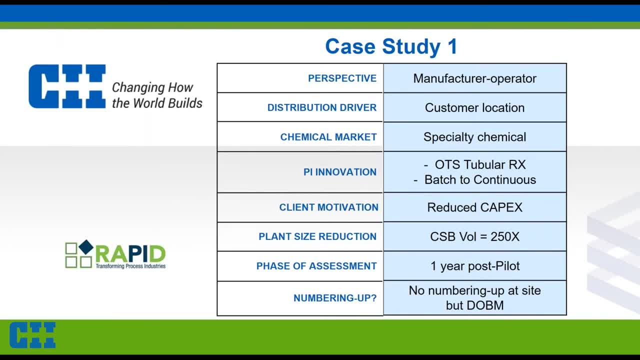 co-PIs on this project. that was all about case studies, So I'll go over case study number one. And also, as he mentioned, we're always looking at MCPI versus conventional stick built. So you'll see that when we start doing comparisons. 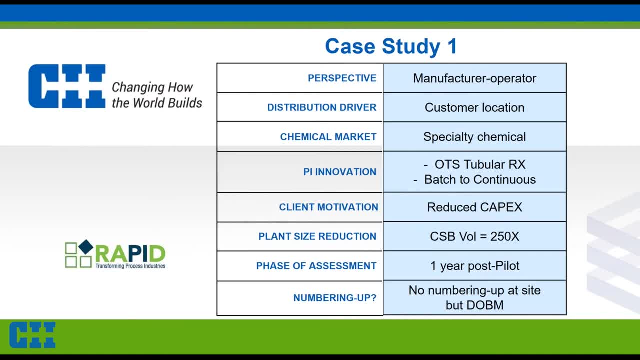 for case study number one, the perspective is from that of the manufacturer operator. The driver for geographical distribution was customer location. The market specifically is specialty chemical. So in that regard, think Low volume, relatively speaking, but high value, So very high value product, but not one that's at a commodity level, for example. 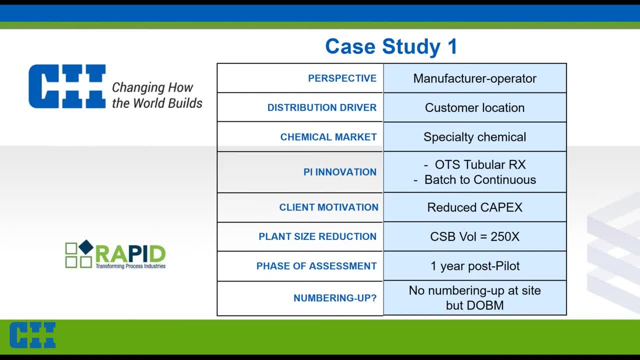 The PI innovation was OTS. That stands for off the shelf tubular reactor and a conversion from batch to continuous. So the conventional stick bill will be a batch approach and we'll compare that to an MCPI Approach- client motivation, primarily capex. 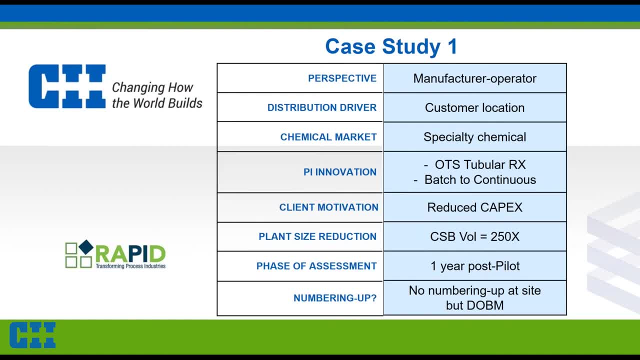 But you know, clients are like kids in the candy store, They like a little bit of everything. And you saw that figure that Ignacy just just reviewed, Plant size reduction- for this case study was was just out of sight. The CSB volume, conventional stick built volume, was about 250 times that of the MCPI volume. 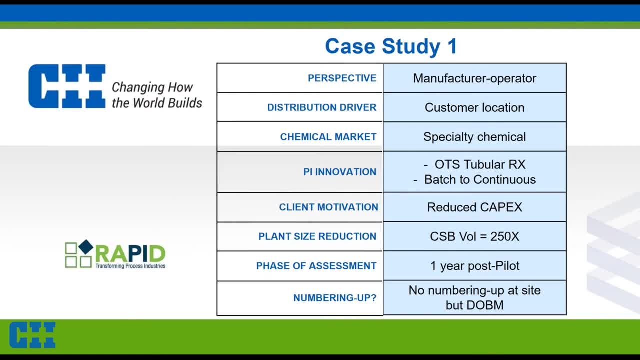 And obviously that represents a lot of material, a lot of piping, a lot of electrical, a lot of structure. So yeah, you're going to see some pretty shocking economic numbers that pair with that as well. Phase of assessment was about one year post pilot. 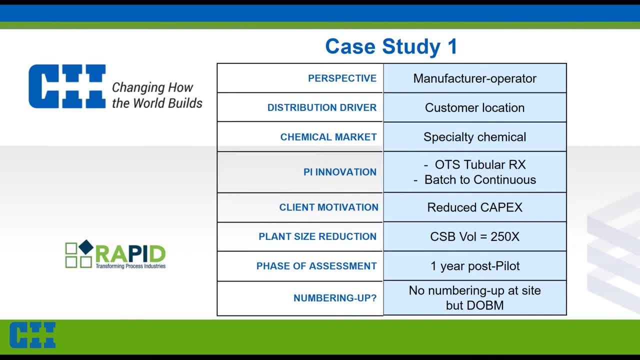 So relatively recent. And then as far as numbering up goes, numbering up is not particularly applicable here, But what we call design, one build, many was, And so the economics of, of engineering at one time come into play. in that regard, Next slide please. 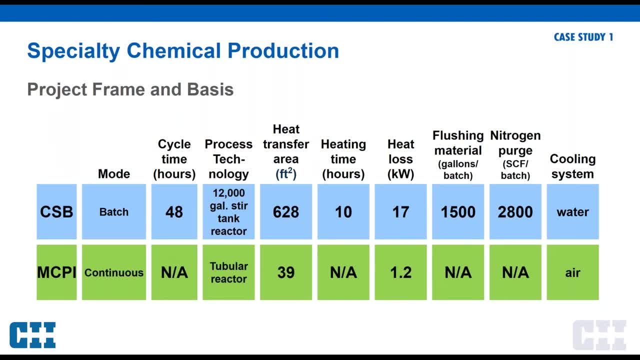 So here's what we call the project frame and basis for some comparisons between conventional stick bill and MCPI. with conventional stick bill We're talking about a two day batch mode, That's a two day cycle, And in contrast to a continuous approach with MCPI, the conventional stick built involved a twelve thousand gallon stir tank reactor. 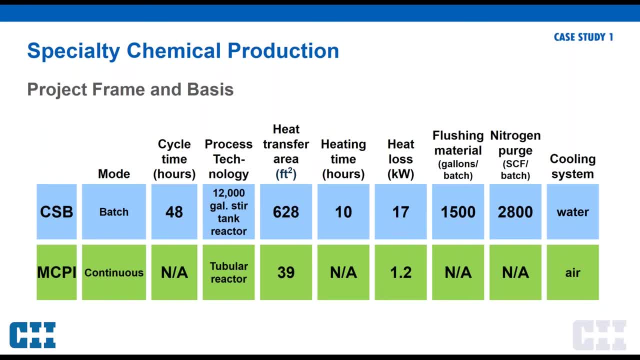 And in contrast to a tubular reactor, which is sort of an all in one solution, not unlike what the example Ignacy provided a minute ago. We then have some heat numbers here in a in a Batch cycle based approach. You know you're turning it on and you're turning it off. 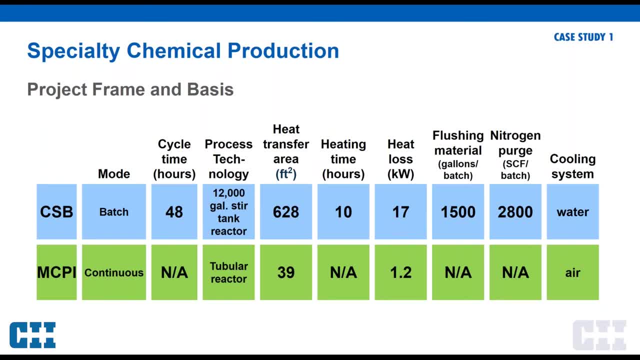 So you have to heat it up and then it cools down, and then you, then you start over again. That's all a little bit less relevant than the MCPI continuous approach. You can certainly see the heat loss numbers were minimal And if you look at the heat transfer area numbers, 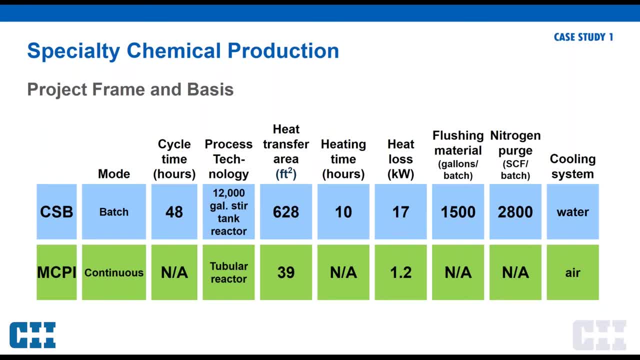 You're starting to see the impact of Process, This intensification, And that that's a factor of 16 right there: 628 versus 39. So that's remarkable. Then you realize that you know when you're done with a batch you've got to clean it up, clean up the system and get it ready for the next batch. 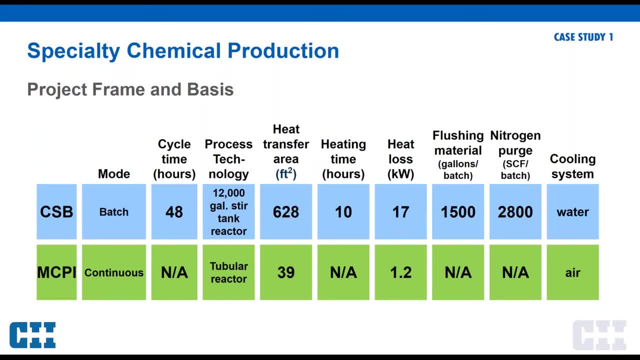 So there's flushing, there's purging. that generates waste, and that waste has to be dealt with. It's not applicable for MCPI. And, lastly, with MCPI, Because of the scale issue, we can rely on air cooling rather than water cooling, which involves, you know, a lot more hardware. 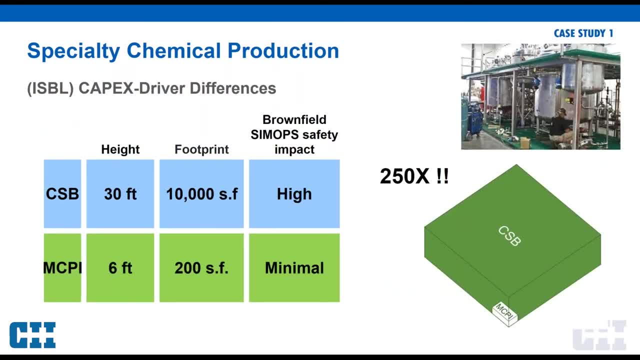 Next slide, please. So, as I said, the the spatial volume difference was radical. So if you look at the green box- that's conventional stick built- You look at the little white brick in the corner, That represents the necessary volume for the MCPI approach. 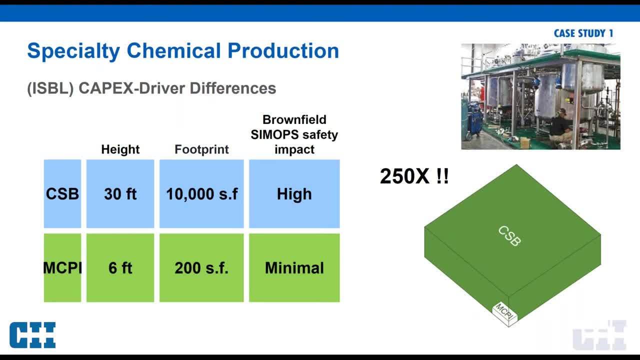 And that's a 250x factor there. The other thing I want to point out is that a ground field SIMOPS safety impact goes from very high and conventional stick built some pretty minimal MCPI SIMOPS, of course being simultaneous operations. 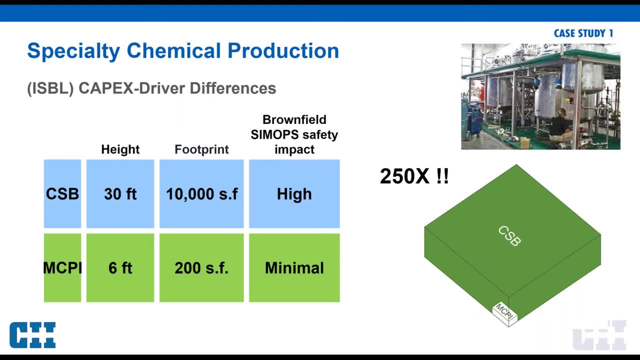 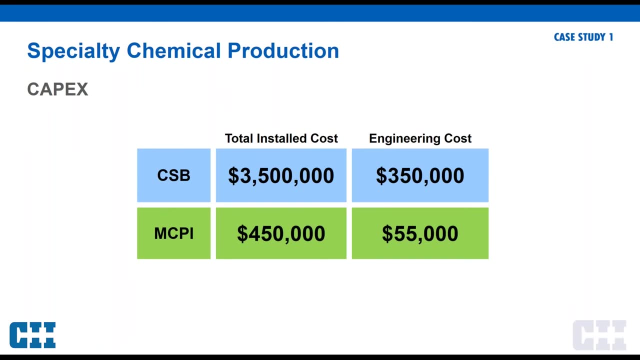 This is where you've got construction going on at an operating plant- Yes, operating plant- and everybody's kind of on high alert because the risks are much higher. safety risks. Next slide, please. So we'll jump to CapEx here on total installed costs. 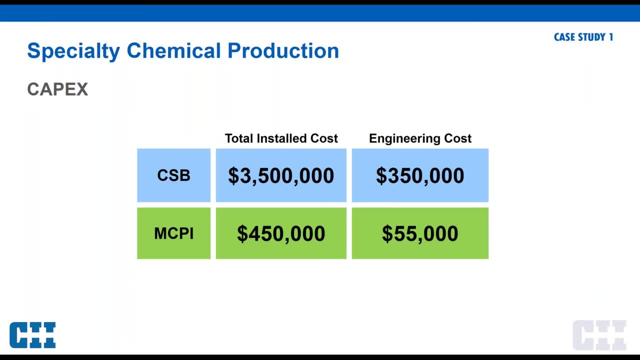 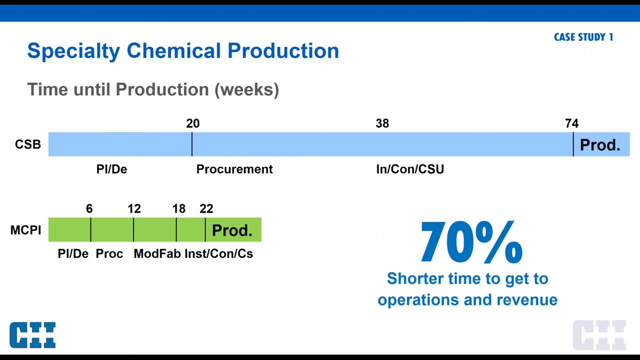 for conventional stick built three and a half million versus 0.45 million. for MCPI, Engineering costs 350,000 to 55,000. So quite a radical shift there. Next slide, please. Here's a comparison of how much time it took. 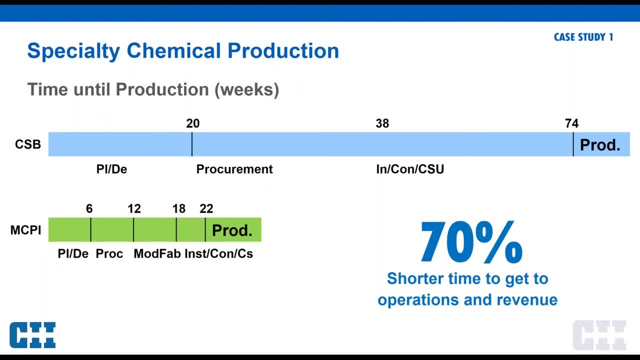 So this is measured in weeks. These are all the various project phases And we can see a reduction from 74 weeks with CSB to 22 weeks to get to production with MCPI. That's a 70% reduction Now in construction. 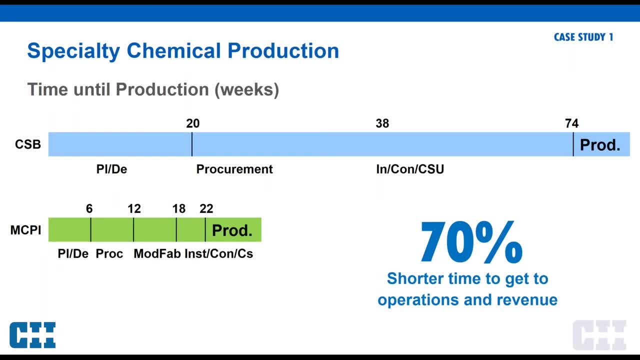 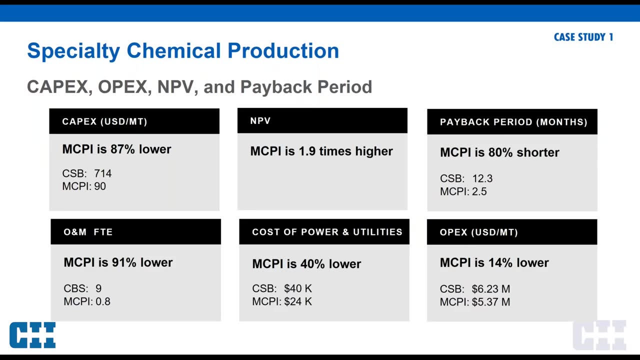 time is money and you just cut 70% of the time off, you're going to save a lot of money with that as well. So that helps explain some of that cost delta. Thank you, Ignacy. Next slide: These are some an overview of economic metrics. 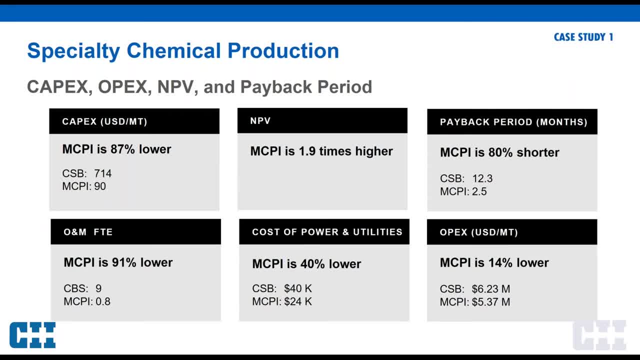 So we've talked about CapEx: 87% lower, NPV almost twice as high, The payback period 80% shorter. Then if you look at OpEx issues, operations and maintenance, full-time equivalent go from nine to 0.8.. 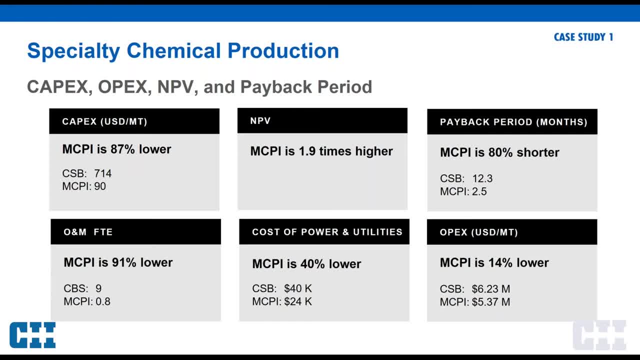 Power and utilities: 40% less. So you weren't turning it on and turning it off, It stays on And kind of the roll up on OpEx itself: 14% lower. The only reason it's not more than that is because you know. 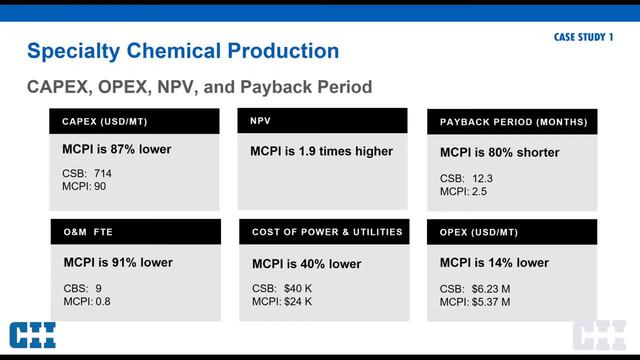 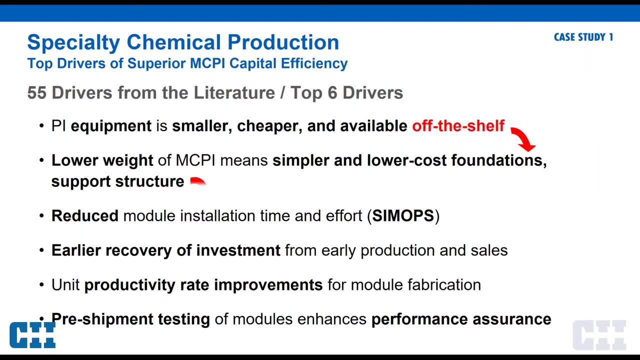 because the cost of feedstocks was quite high for this product. Next slide, please. From literature and from interviews with industry, we identified 55 drivers of cost or some other benefit and presented these to each of our case study project managers. they identified the ones which they felt were most relevant, most significant, and these are the top. 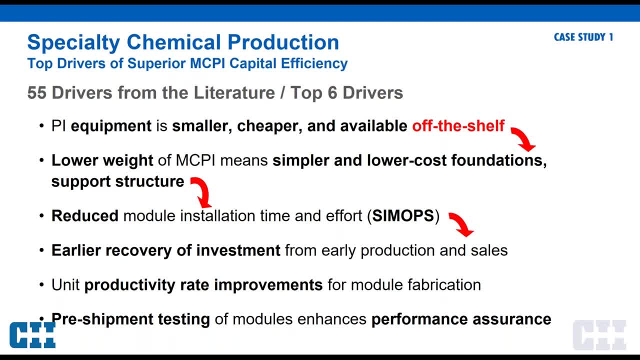 six drivers for this particular case study. so we're not generalizing this across all mcpi applications, but we're saying these are applicable, highly applicable for this particular case study. so pi equipment: smaller, cheaper, available off the shelf. lower weight, simpler, lower cost foundations and support structure, as i said, the reduced um installation time and the sim ops that comes with. 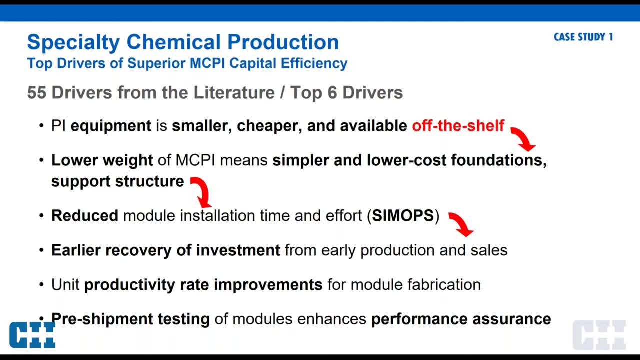 that earlier recovery of investment unit productivity rate improvements for module fabrication- so it's a kind of a classic benefit from shop fabrication- and then pre-shipment testing of modules enhances performance assurance, so more likely that things will work when you get it out in the field. before i hand it back to agnasi, i just want to mention a couple other points that are included. 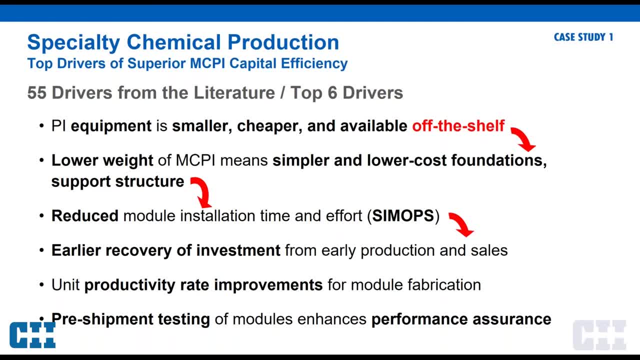 in the report- by the way, the final report it's fr dash 373 for those of you that are cii member- with member companies. the first uh point to make is that we found that, given the the high profitability of this particular product and the low capex cost, 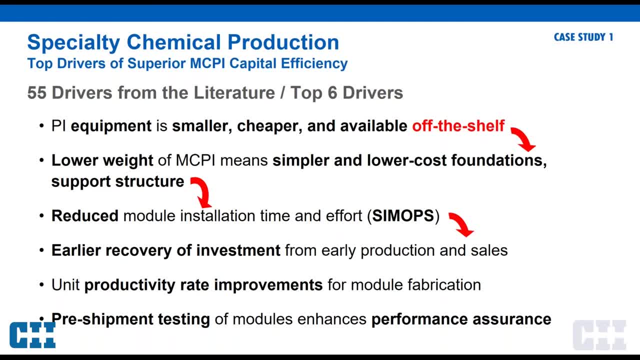 of the mvpi that it actually makes sense to invest in a second redundant backup unit just in case there's downtime, and those economics were highly favorable. the last point i want to make comes back to the process safety issue associated with hazardous fluids, as indicated by the quantity. 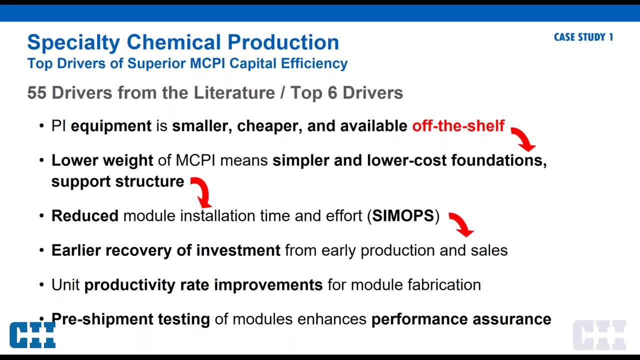 of fluids and so we we talked about that 12 000 gallon situation and how much of that total weight is included in the 100 to 100 square meter of the mcpi. but the the size of the mcpi approach is about 30 gallons, so that's a 400x reduction. 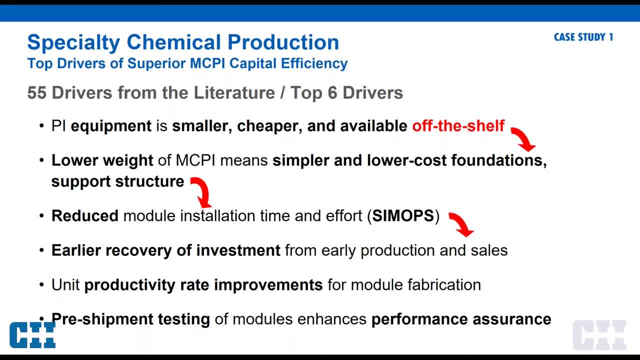 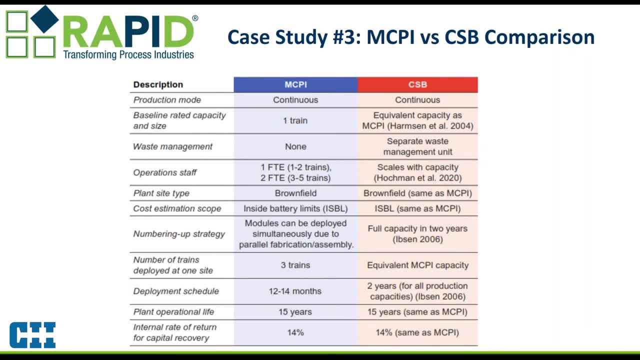 in in risk exposure. so with that, i'm going to hand it back to agnasi and he's going to talk about case study number three. all right, thank thanks, jim. so so case study number three is a bit of a a a real eye-opener because of the huge benefits that the MCPI approach shows. Case study number 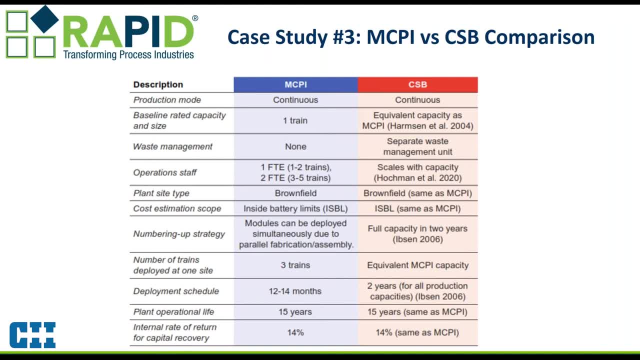 three is really one of those that the preconception is always that for a commodity chemical, for a large volume chemical, a centralized, what we call that CSV, that conventional stick-built approach should be better. It's expected to be better. So let's put some numbers behind it And what you 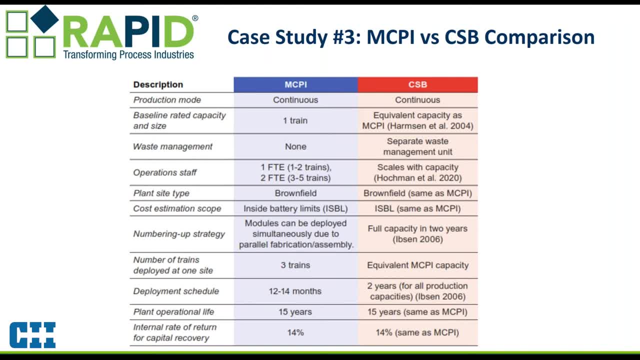 see here both the MCPI and the CSV approaches in this case is continuous. The issue becomes on number of trains versus capacity. Obviously, on a centralized approach the way you get capacity is by having a larger plant. On an MCPI approach, you have more trains, right. 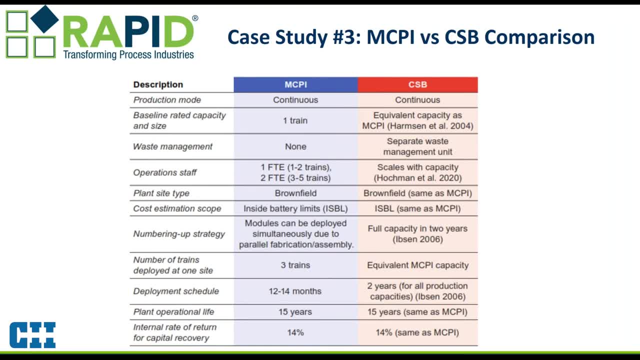 Still you have that advantage of the deployment schedule on the MCPI size being able to get to scale in a more step-by-step approach which allows you to get to some scale faster In this case, obviously, the operational lifetime and rate of return. 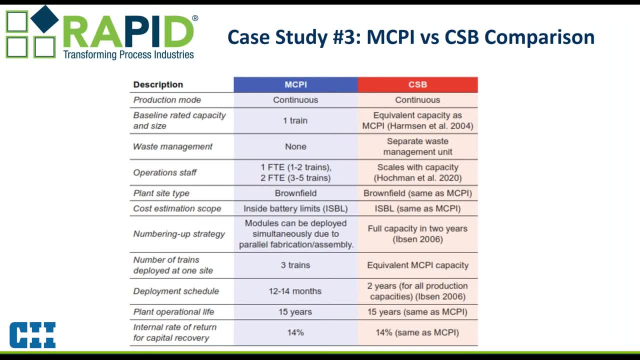 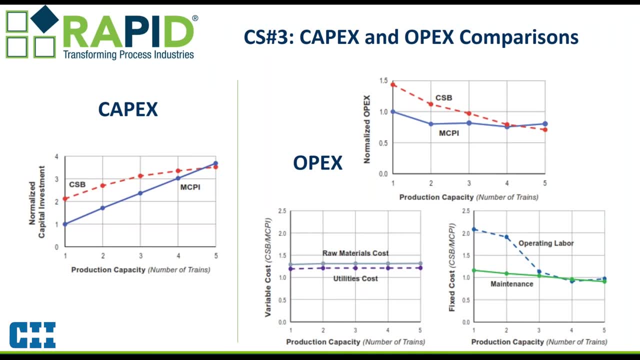 were put at the same level. to be consistent and to have a bit of a fair approach, I will jump directly into some of the CAPEX and OPEX comparisons with this plot. On the CAPEX side, what you see is sort of what should be expected, right, Which is: 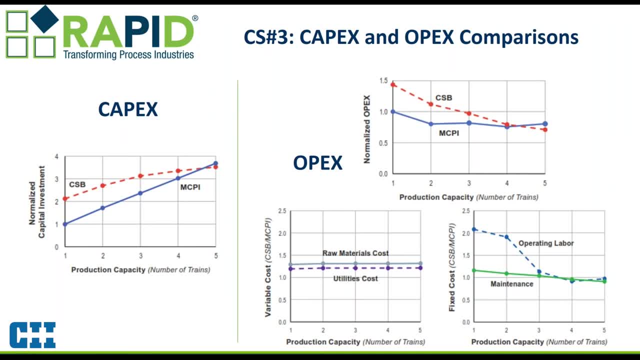 the MCPI approach, which is the blue line in there on the left. It's a gradual increase right. The more trains you have, the more capacity you have. the more capacity you have to get to the MCPI, The more it goes up. So you have a bit of a linear increase with the number of trains. 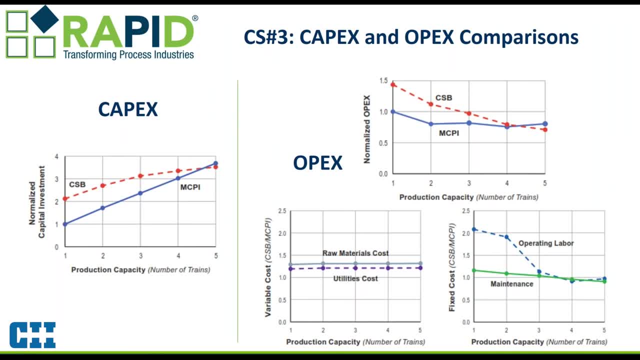 While in the stick build, what you see is a curved approach, a curved growth. but it kind of peters out So right, The more trains you have, or equivalent trains you have, the lesser the advantage of the MCPI approach. So clearly on a CAPEX. 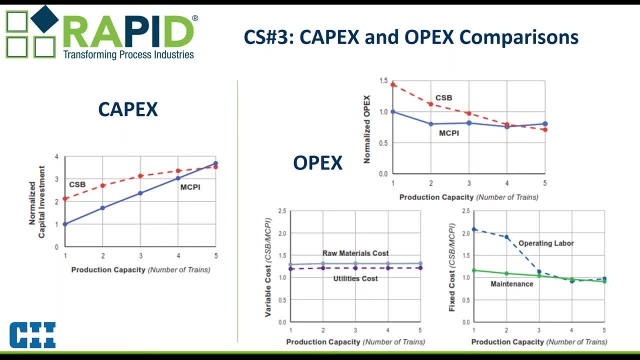 perspective, if we're going to have one, two, three, a number of trains, there is an approach, there's an advantage, a clear CAPEX advantage, at going at it from a modular, intensified approach. At four, I would say you're sort of getting close to equivalent, and five is really you know. 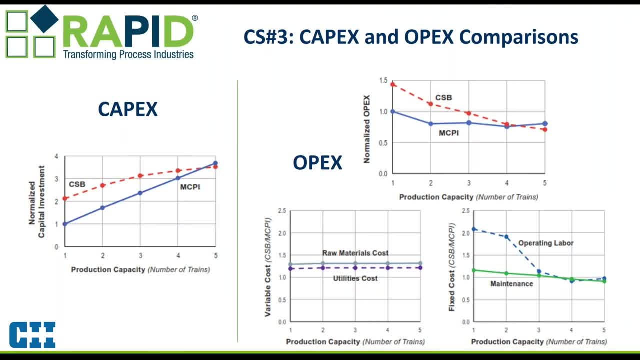 crossed the other way, And if you were higher than that, the stick build. the centralized approach clearly starts winning out. So this is what we, conceptually, we would be expecting In this case. that crossing of the lines is in that. you know roughly four and a half idea, so that we see that. 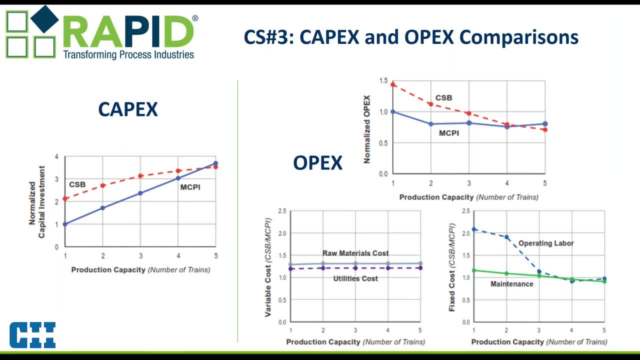 there is a good range for production capacity at which MCPI has an advantage before a stick build takes over. Looking at OPEX, you see something not too different, but it's important to look at not just the total normalized OPEX but also what goes in there right. So when you look at utilities and raw materials costs. 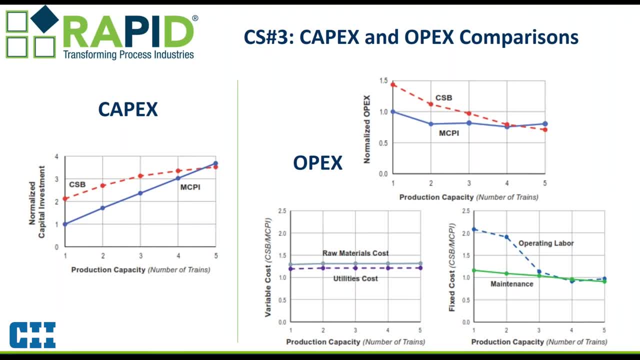 so those variable costs, what you see, that that's obviously kind of proportional to the capacity, so that there is no real advantage or very small difference between the the two approaches. You see there roughly the changes. there's no change in capacity between both of them and their slight advantage to one of them. 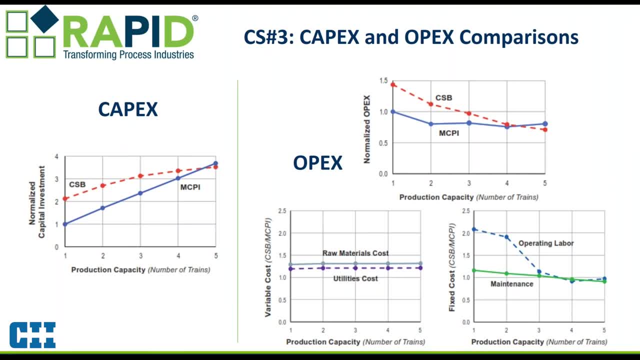 When you start seeing more of a difference, it's on fixed costs, right? So fixed costs, especially on the labor costs for underutilized, larger plants, the advantage of the modular becomes higher, right? So that idea that it allows us to scale up more stage by stage means that we don't have extra labor because we have a centralized plant. 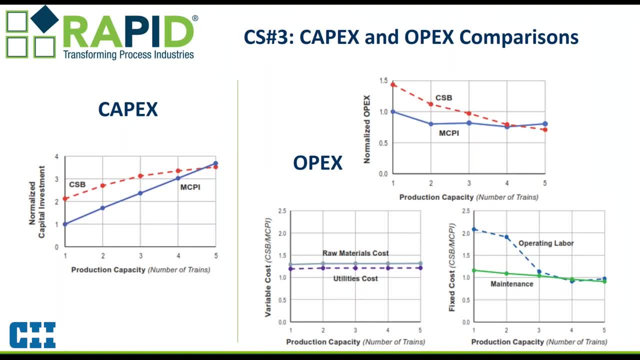 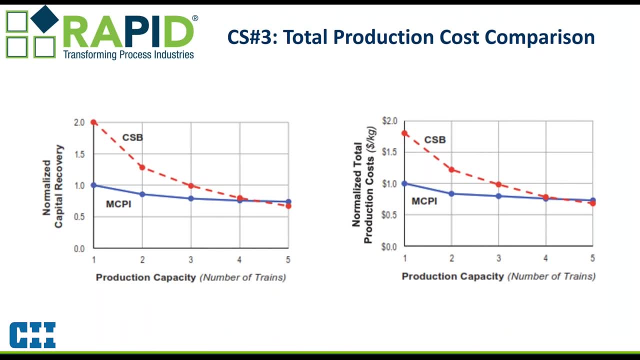 So we put CAPEX and OPEX together in a more total economics and total production costs, We see what we would expect, right, So that for lower number of trains, and in this case the cross point for the combined is roughly at that number of four trains. 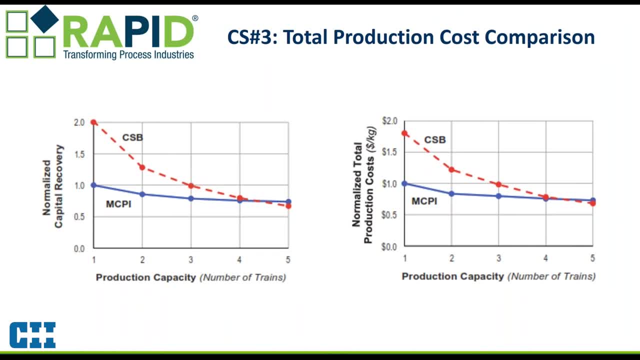 There is an advantage of MCPI. The more trains you have the advantage of MCPI, so lower capital recovery or production costs. You see the shape of both curves being virtually identical. So production costs an advantage of MCPI. until you get to that four number of trains in which you get basically equivalent. 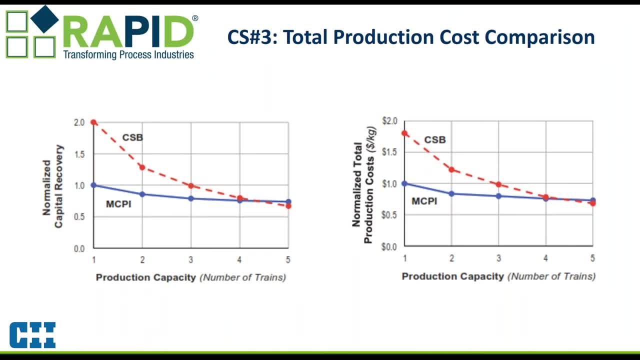 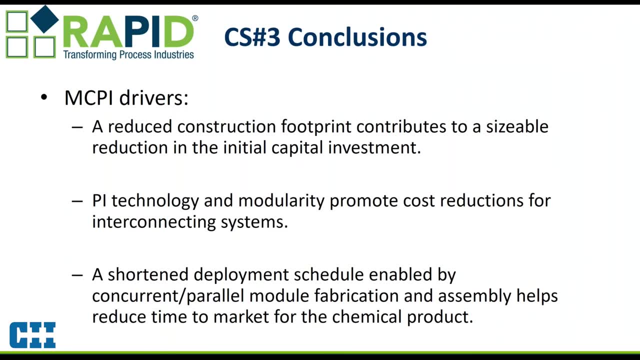 And crossing that stick build the centralized approach starts sticking Yeah, So that's one of the main advantages. So what are the MCPI drivers that we see from those results? So that reduced construction footprint makes a sizable reduction in the initial capital investment right. 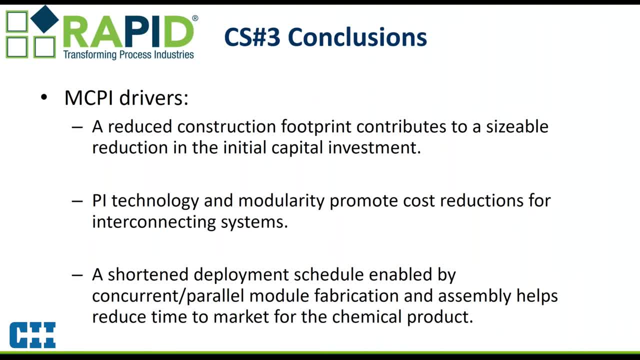 So that initial investment is much less. You don't need to have because you're able to do that module by module. you don't need to have the whole capital. You don't need to have the whole capital available at the beginning, which gives a career advantage. 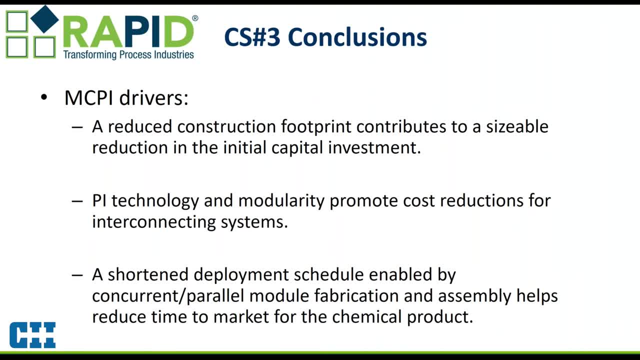 The cost reductions, especially on the CAPEX side for the PI and modular technology for the MCPI, are really driven by the interconnecting system by piping and similar wiring type of approaches. And then we also see that a lot of the additional So what are the advantages? The cost reductions, especially on the CAPEX side for the MCPI, are really driven by the interconnecting system by piping and similar wiring type of approaches. The cost reductions, especially on the CAPEX side for the MCPI, are really driven by the interconnecting system by piping and similar wiring type of approaches. 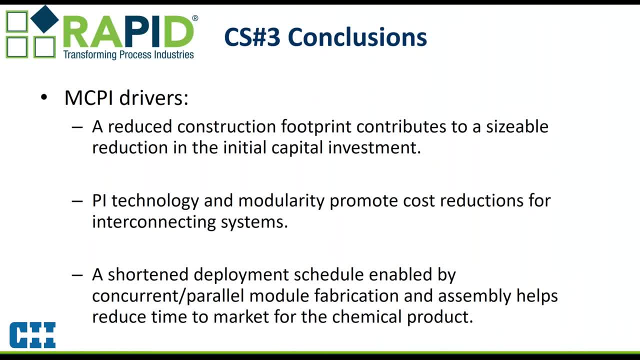 Come from that shortened deployment schedule that Jim referred to before. So the ability to do parallel and concurrent module fabrication and assembly really helps. right, You can do it. You can build the different trains at the same time without having to have an all or nothing type of approach. 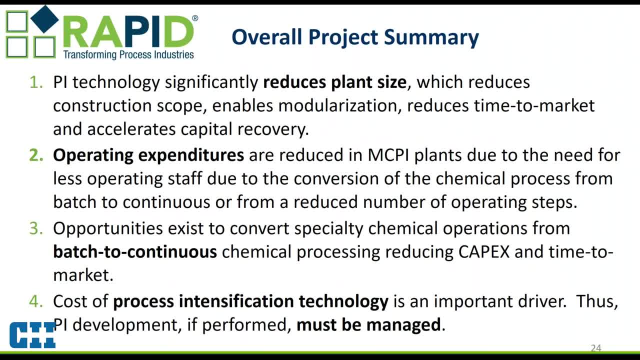 So from an overall project- And this is going beyond case 1,, 2,, 3,, 4, when you put them all of them together and kind of look at the overall conclusions, this is kind of the main conclusions that are spelled out in the report. 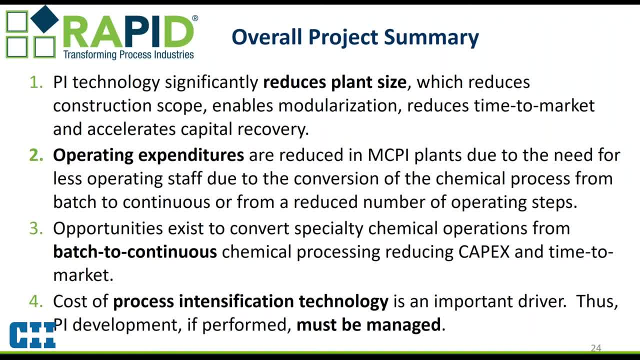 that Jim just made reference of too and I'll talk to a little bit later as well. So PI technology, so that the intensified side- not yet the modular- really reduces plant size. right, And that's a critical point, Intensification really enables modularization. 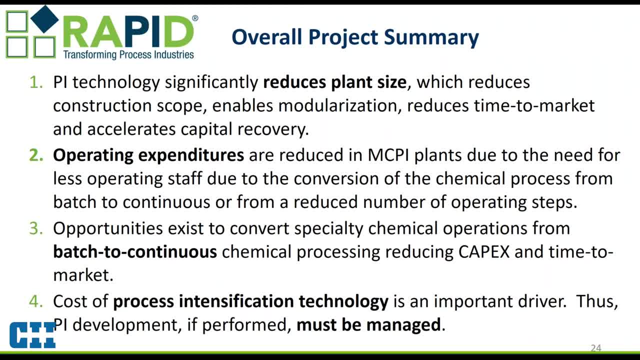 A modular approach without an intensified technology is a very limited scope. So intensification enables modularization, reduces construction scope, reduces time to market and really accelerates the capital recovery. right, We start producing and getting revenue quicker, so we start paying off the capital quicker, and that's a huge advantage. 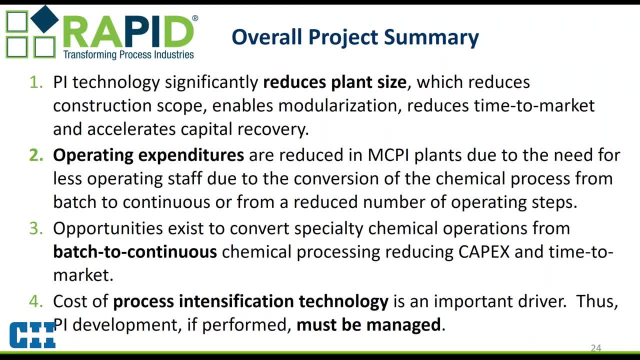 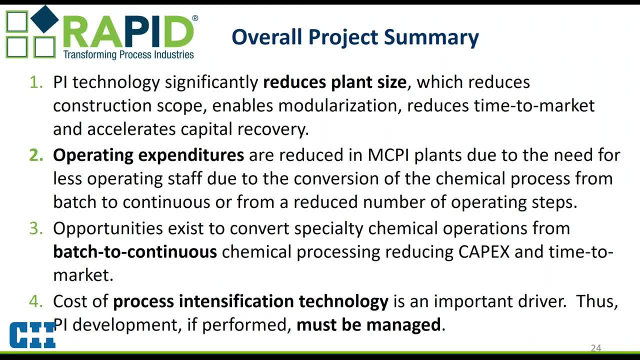 steps BATSU continues is really a key opportunity for MCPI to show its full advantage, especially reducing capex and time to market. You saw from case study one that Jim presented, the huge advantages for those types of opportunities, The cost of process intensification. it's an 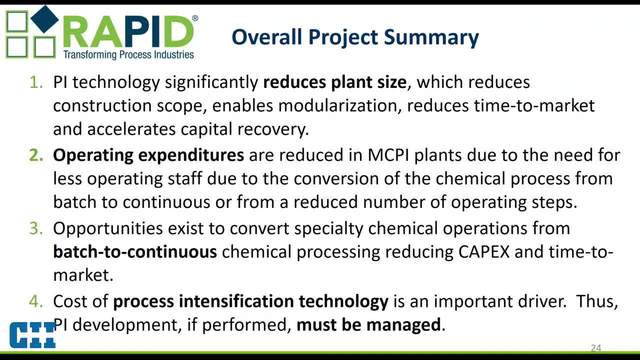 important driver, So it must be managed appropriately. And there is a number of conclusions, more detailed conclusions if you read the report in which it's important. for example, I'll bring one of the ideas, which is go after off-the-shelf technology or 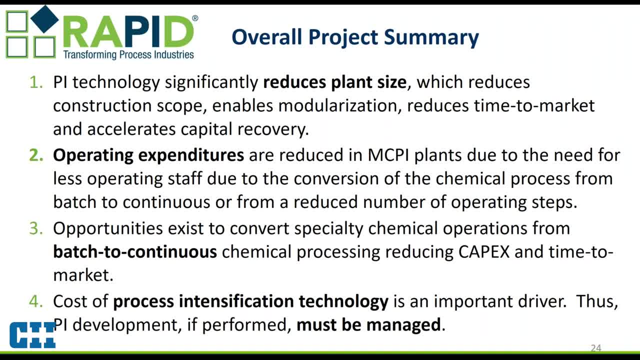 off-the-shelf equipment when intensifying Custom-built equipment. custom-built equipment is always always more expensive and it can eat off some of the savings. So important to understand where the pressure points are, where the advantages of both approaches are, and then take full. 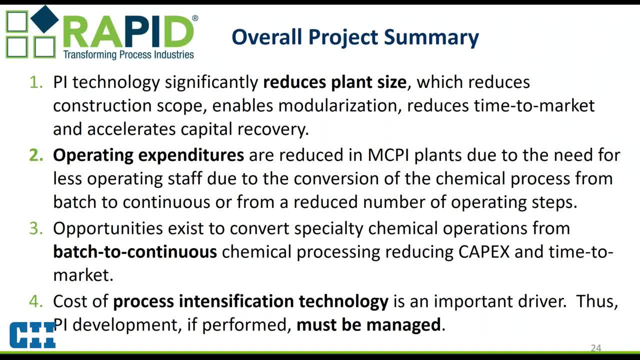 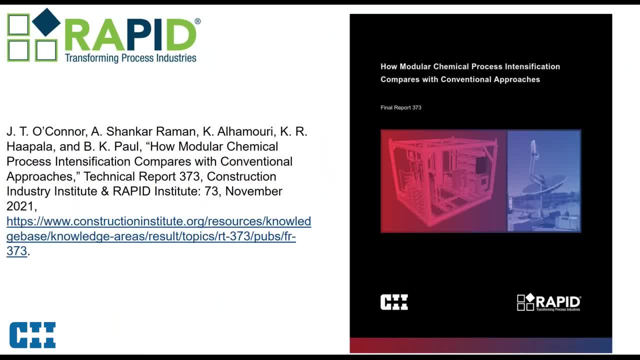 advantage of them for the cases that they are appropriate. So I wanted to kind of go towards the end of the presentation and then pass it on to Olivier. This is the report that Jim made reference to, Final Report 373 in the CII world. This is available to both CII and. 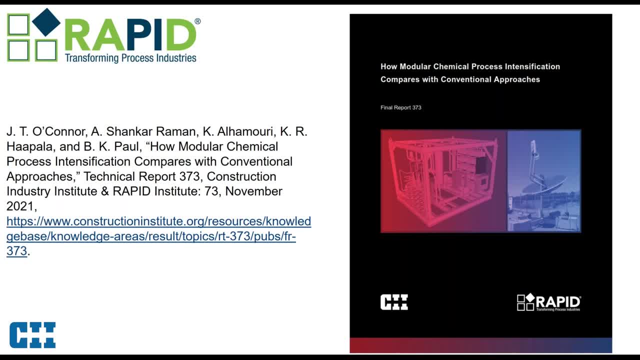 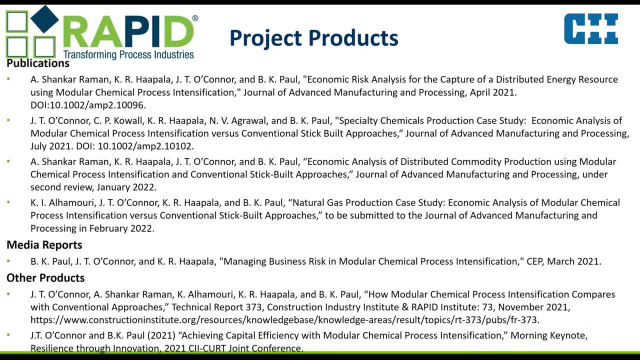 Thank you, Olivier. Thank you, Olivier, Michael. if you have many questions or interest in seeing the status result of these这么 and Cem report seven, I do not. I need to Go ahead and select a grade. Ah, Go ahead Next slide. 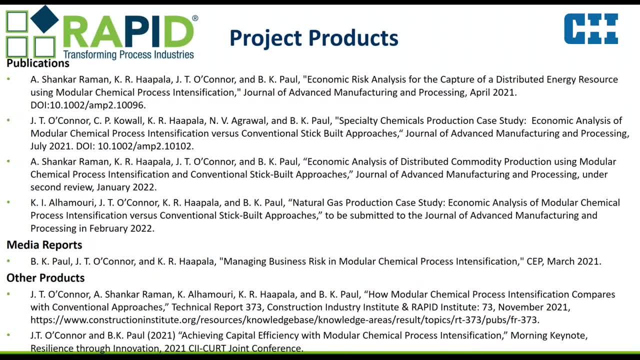 the conference last year. There is also an article that Brian Jim and Carl Hapala from OSU as well, wrote in CEP. CEP is the magazine that all AIC-HE individual members receive, so March 2021 available. And then a number of peer-reviewed publications, mostly in the Journal of Advanced. 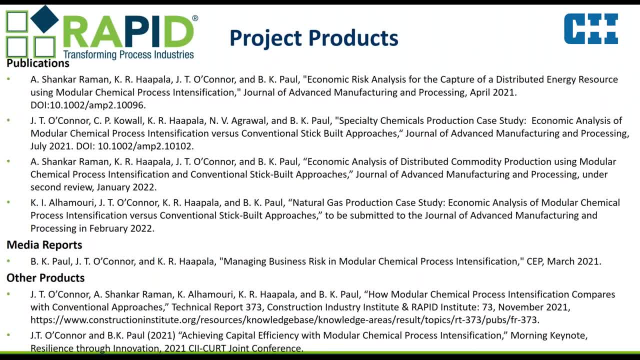 Manufacturing and Processing, which is a widely publication and is the official publication of the Advanced Manufacturing and Processing Society, a community of AIC-HE. So this is a peer-reviewed publication. A number of these four articles or papers have been already published and think 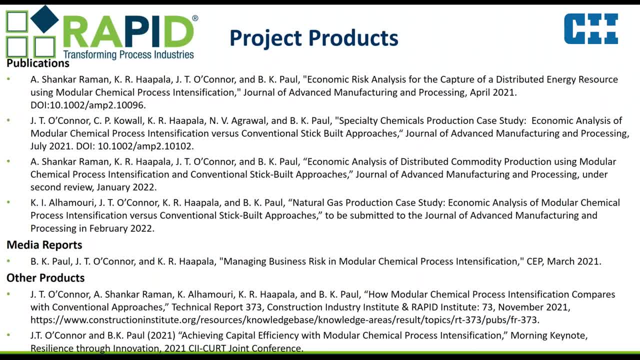 there's a pending one. So those of you who want to look at details on the cases, you know a number of things That can be looked at. So I'll move it on to Olivier. some thoughts on CAPEX and then close up. 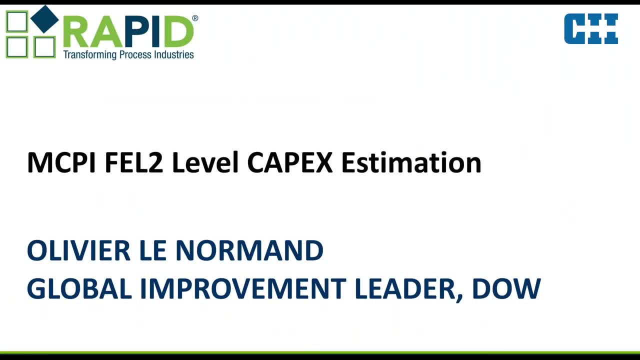 with some high-level conclusions, Olivier. Yeah, thanks, Ignacy. So yeah, I'm Olivier Renormand, working at Dow Chemical as a global improvement leader, And there I mostly look at, you know, modularization in our CAPEX portfolio. So what I'm going to talk about here is just 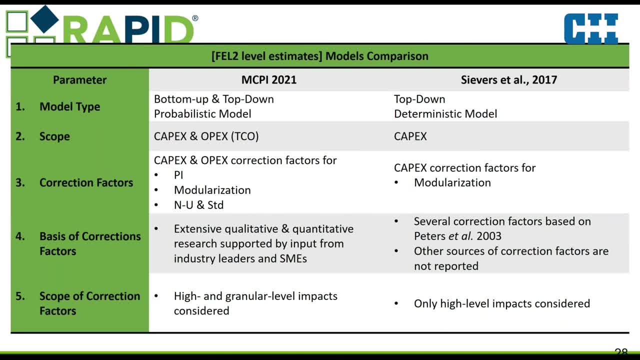 another aspect of this study that was led by Jim. I came in this study as a member of CII and tried to help the best I could. I just barely have enough knowledge to be in this webinar and present what I'm going to show, So I'm going to start with this first one. So I'm going to start. 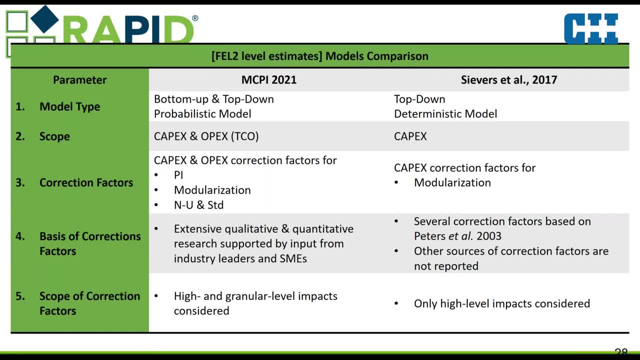 with the first one. So I'm going to start with the first one. So I'm going to start with the first one. Let me show you here. But in summary, the team developed a cost estimate that I think can be useful for owners, but as well engineering companies, EPC companies, to evaluate the value of 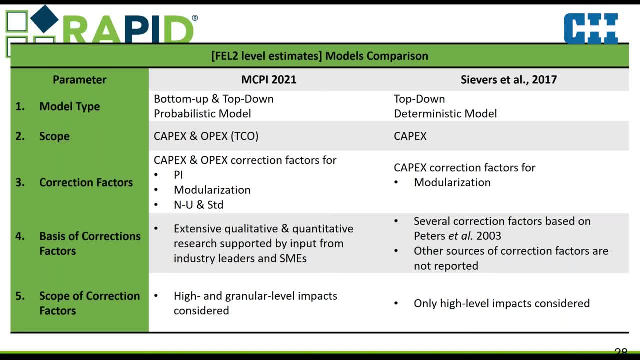 MCPi at this time when you don't have enough data or project yet and you want to know if you are going or not to develop- Yeah, modular, but maybe more modular- and process intensification really a key element here. so this mcpi 2021 cost model was developed in the frame of this effort here and you see a table here. 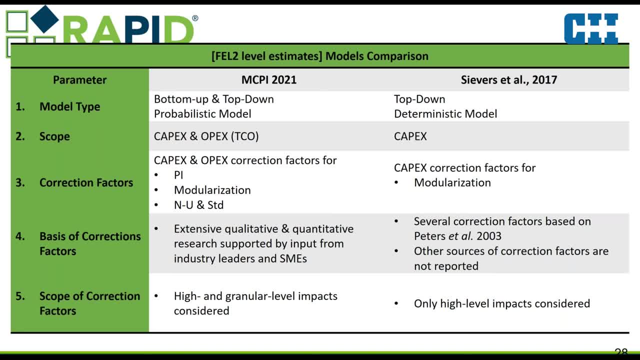 showing how it was developed. what are the main characteristics of this cost estimate? and it is compared to another model that apparently the the research team was, let's say, benchmarking against. that used to be one that modeled the cost for the impact of applying modularization only, which is sievers. model type is bottom up to top down probabilistic. 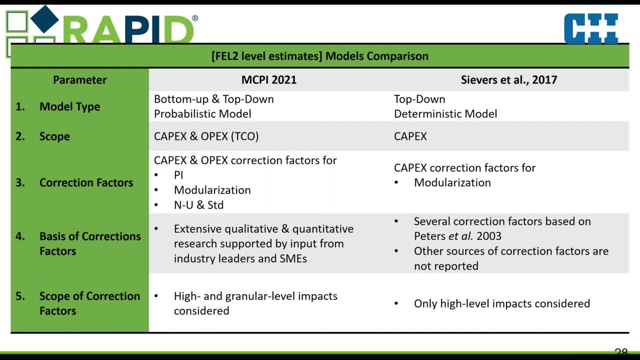 model. so to me that means it's based on, it's a factored approach, if you want. so again, high level, and i think it applies to fel2 level estimate, maybe a field one as well for everyone. fel means front end loading, and they feel one is really about project definition. 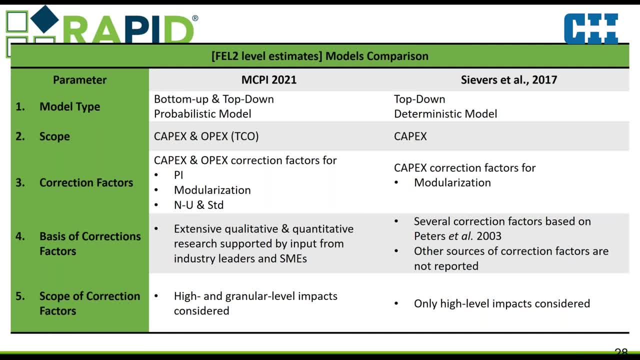 the field. two is when you start to define your scope, so you see the different elements that are part of here. i think, on element three, correction factors- which is really where the know-how was put into place in terms of when you are applying, whether you apply processing into the identification. 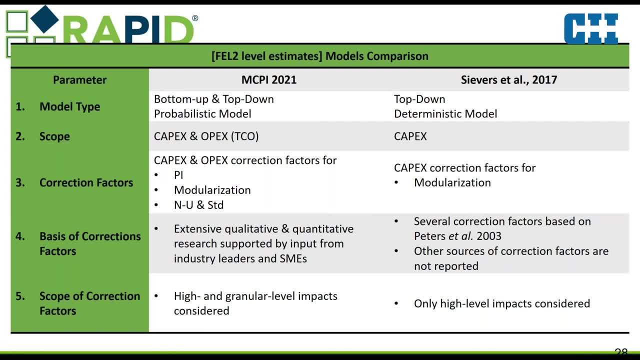 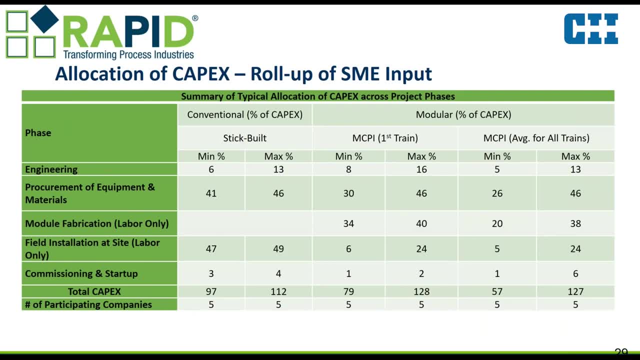 motorization and numbering up as well, so there are set of different factors for each of those elements. i think we can go to the next slide, so we are participating in this, in this research, we were asked to trying to do two things really: What is the allocation of CAPEX? and we looked at OPEX as well. 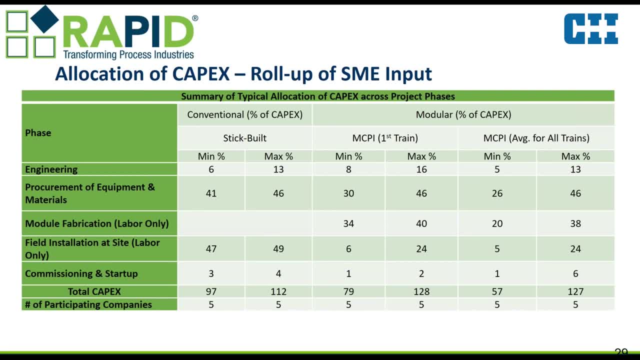 what is the allocation of CAPEX within different categories, which you see on the column on the left: enduring procurement, fabrication, financation, and all that for conventional stick build. so that's the two other columns, and with a mean and a max. 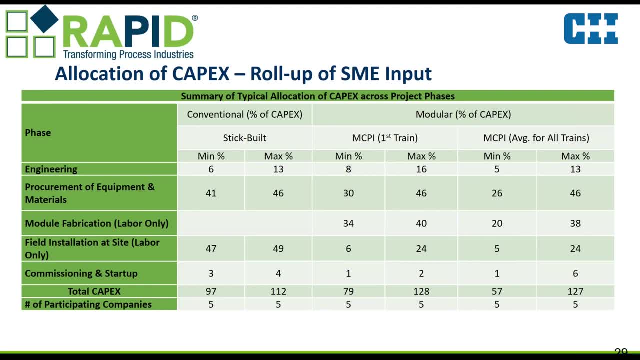 which gives you this probabilistic approach as well to the model, and then have the same allocation distribution for MCPI, which are the four last columns, and you see the distinction between one train or the first train and then the following trains, when you do number up. 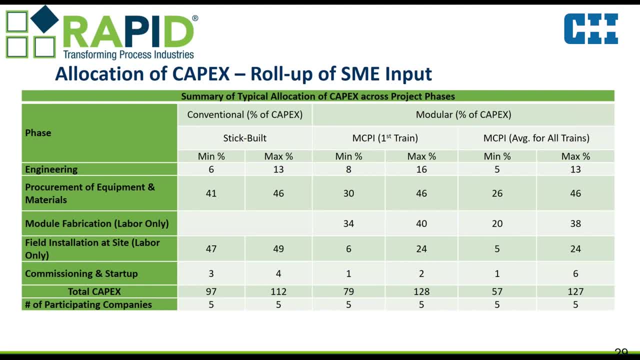 so different allocations and really what before showing the next slide? the next slide will show you the correction factors or the impact of modularization process, intensification and numbering up, but what you would do is, if you know your CAPEX for your conventional stick, build. 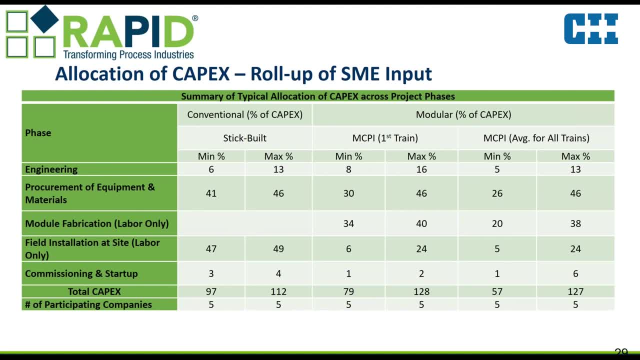 for the facility. then you can take this number, break it down back into either MCPI one train or MCPI- you know different trains in the way it is shown on this table- and then go to the next table, the MCPI one, and then the next, then the next and then the next. 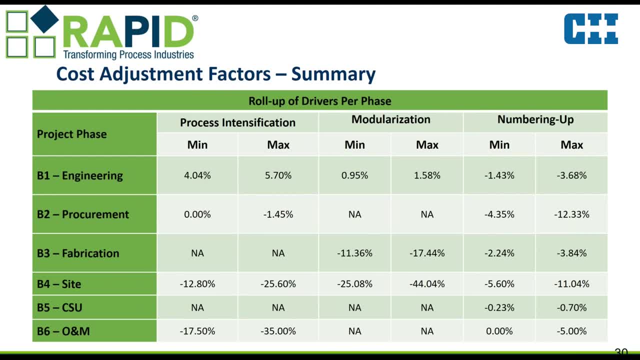 and the next: The next table, next slide, which shows the adjustment factors that have been determined by the research team and the input from different SMEs and people from the industry, CII members. And here this time the correction factors are applied to those different B1,, B2,, B3,. 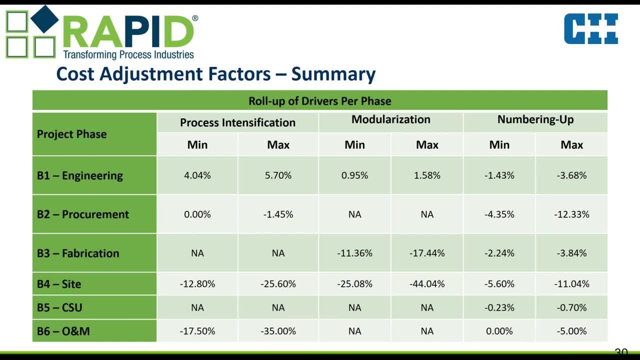 six categories, and then you would have an estimate of the capex for your MCBI project, which I find beautiful. Now the question is: does it work? So the research team didn't study it. from here and going to the next slide, they have tested their model against. 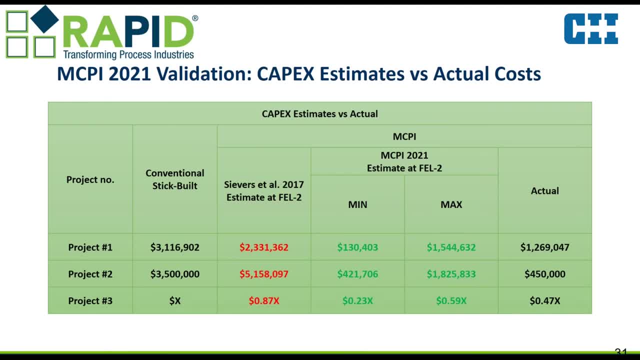 those case studies that you have seen, which are real case studies and for which they have the actual cost. So on the left side you see project one, two and three. I'm not sure they correspond exactly to case one, two and three, but I don't think that's the propose here. but you have 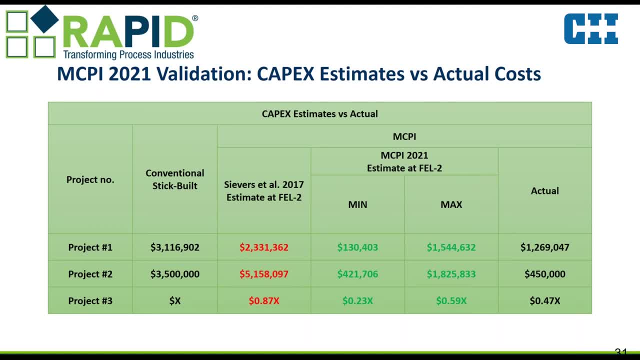 the conventional stick, build value, against which we make the comparison, and then you have in green those mean and max for the MCPI, using the cost model I showed you on the two tables before and you can see how it compares to the right column which is actuals, and looking at that, I mean you would see that. 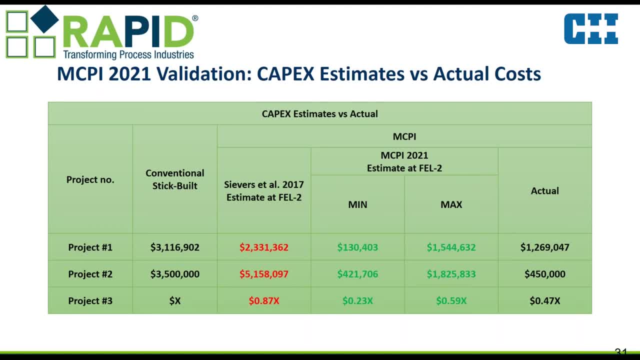 it's really not that bad, and honestly I didn't think that would yield such good results. but I think it's pretty good, and so kudos to the research team for having done that. I think that can be a useful way of approaching the question for the industry. 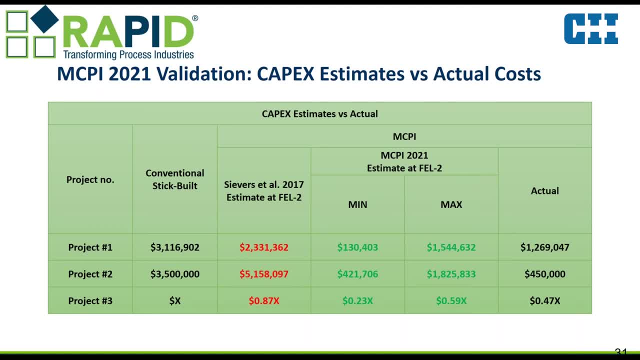 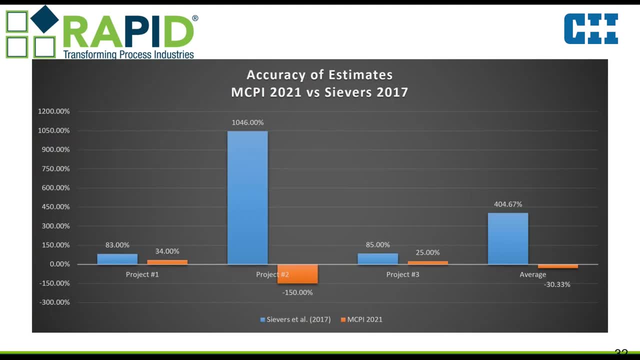 And to decide whether or not it should grow or not with the MCPI. I think it's a good start. The next slide shows the level of accuracy obtained with this model. Blue is for the other former benchmark cost model, but in orange, you see, for different projects. 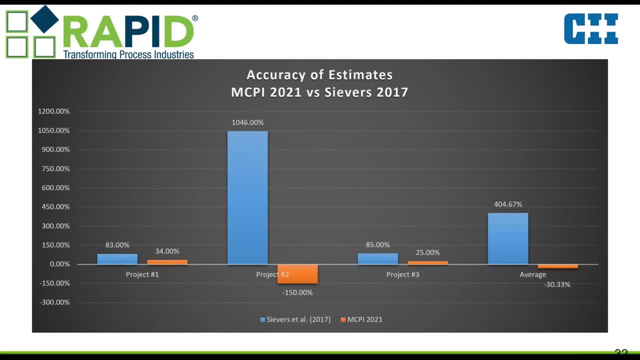 how the cost model accuracy was against actuals and you see the 34 percent, you know: 25 percent for project three and 30 percent accuracy for project overall. One project was a little bit off but of course everybody needs to understand that there's. 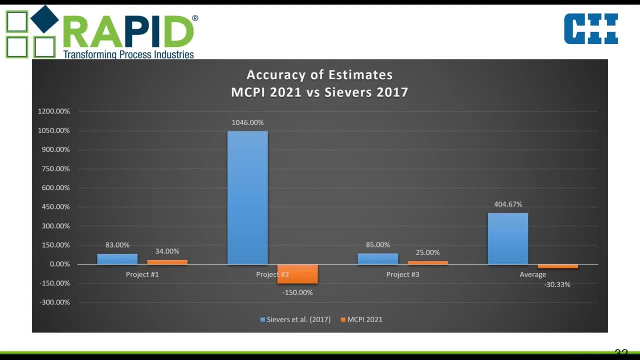 no one model fits all. you know, one solution for all. but I think those correction factors can also be tuned depending on a specific project. So I think that's a good start. So I think that's a good start. So I think that's a good start. 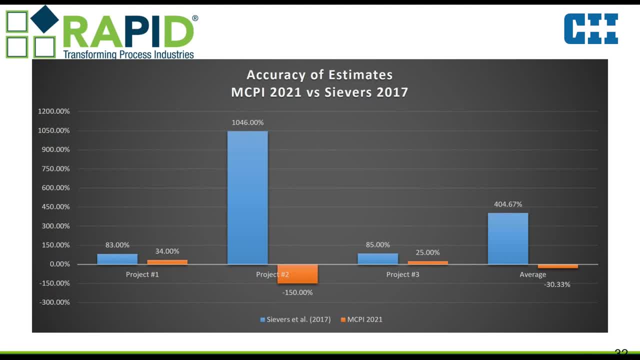 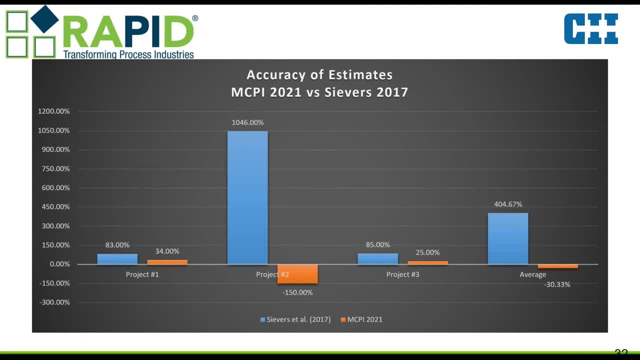 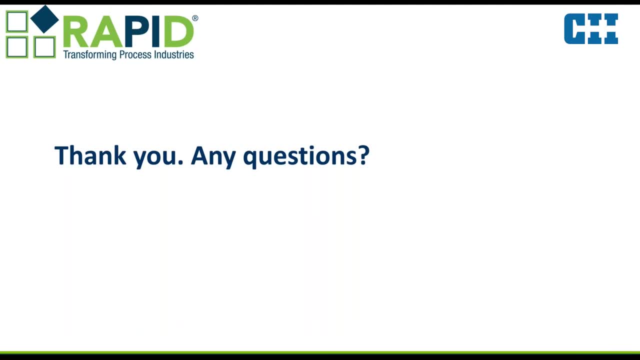 That's all I had to share on that back to you, Ignacy, Thank you. thank you, Olivier and Jim. I think this is kind of the end of the presentation. I thank you all. I just wanted to give another plug. 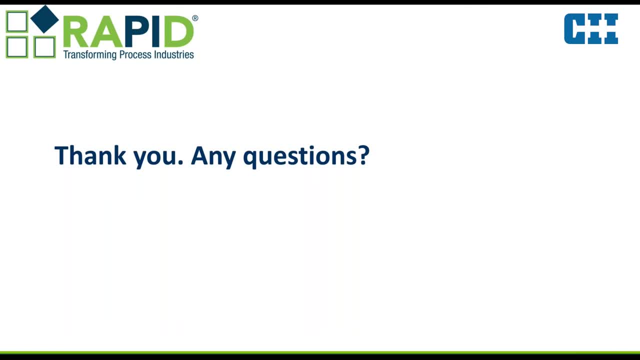 I think this is kind of the end of the presentation. I just wanted to give another plug. We would like to continue some of this work. We have these four cases. as you saw, they are somewhat scrubbed from identifying data. they're all are real cases in which, or you know, the data was collected. 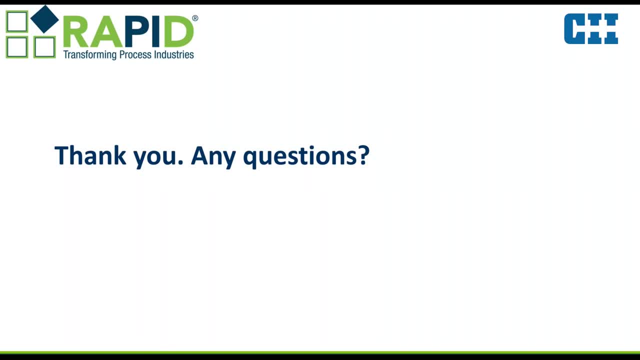 through interviews and through, you know, work in collaboration with, with the companies involved, but the presentations, the sharing, was a scrubbed of that. some of them are much more or less identifiable. we would like, and do, reminded me yesterday of that, finding, you know, a fifth and a sixth case up to 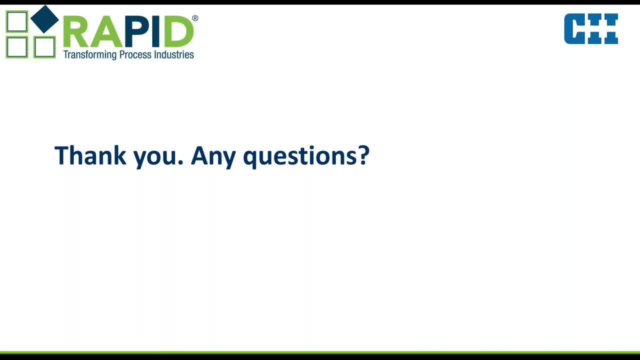 potentially have a wider coverage of the process industries in the different cases and really understand the potential value and plus and minus value of of these modular intensified approaches for new plants or for Brown and Greenfield. so if you guys are interested, any questions, please feel free to put them in the Q&A box and I'll see you next time. 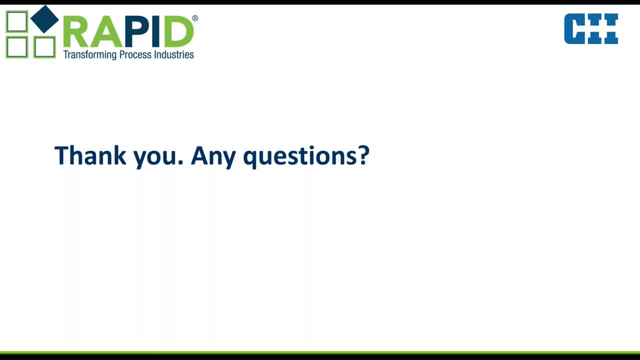 anybody you know. contact any of us and we will. we will. we will work with you. we'll try to figure out how to best incorporate it. so thank you. I think we have a little bit of time for questions. but yeah, Ignacy, if you could advance to. 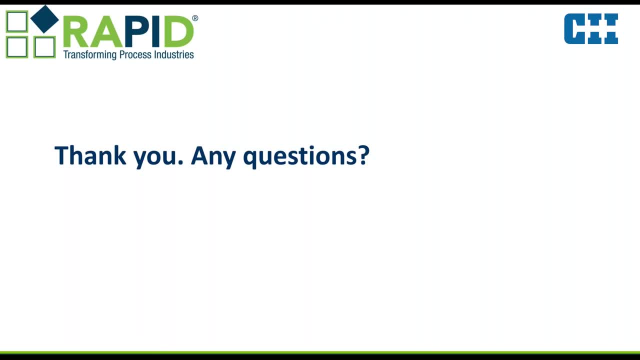 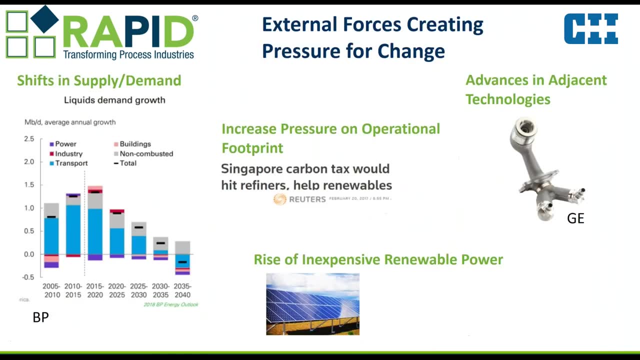 the next slide that'll give the contact information for folks to reach out. I think I had some final ones. I don't see the final. I think the very last slide had some contact info, maybe not? I apologize, well, I am not showing you the contact information for the next slide. I apologize, well, I am not showing 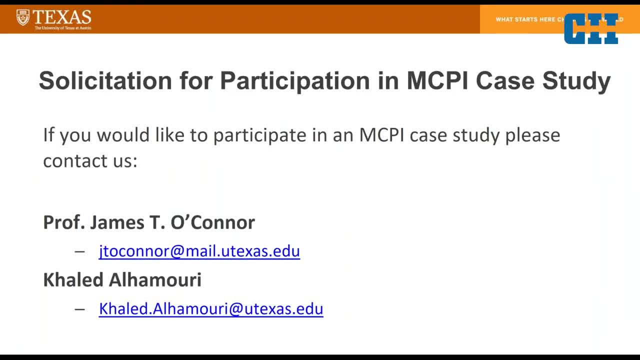 well, I am not showing you the contact information for the next slide. I apologize. well, I am not showing any. there we are. oh, there, it is fabulous. so if you guys do have any need to contact Jim or Ignacy or Jim's assistant here, you can certainly. 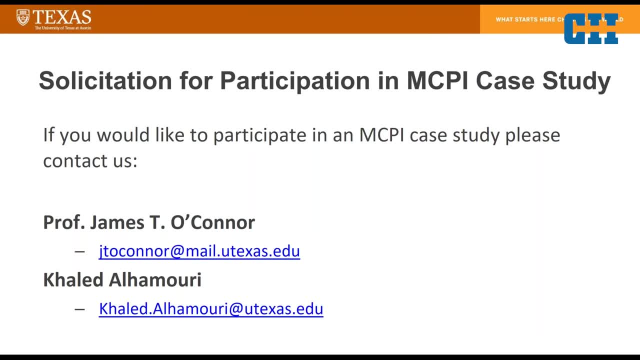 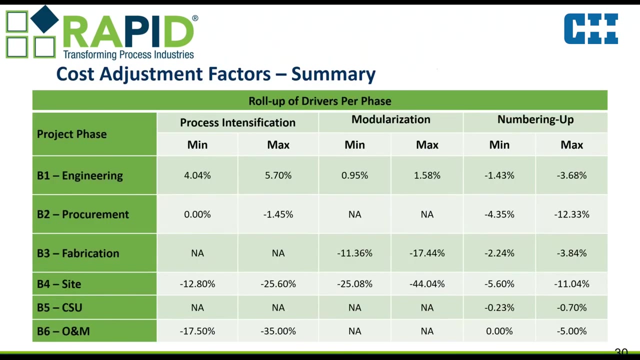 approach them via those email addresses. we'll get you in touch with Ignacy as well. I am currently not showing any. oh, we do. we have a question here. did you study any brownfield projects? yes, yes, we did. I mean it technically speaking. the case study I went over was: 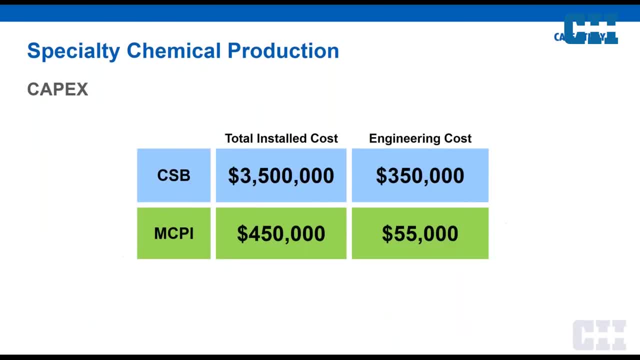 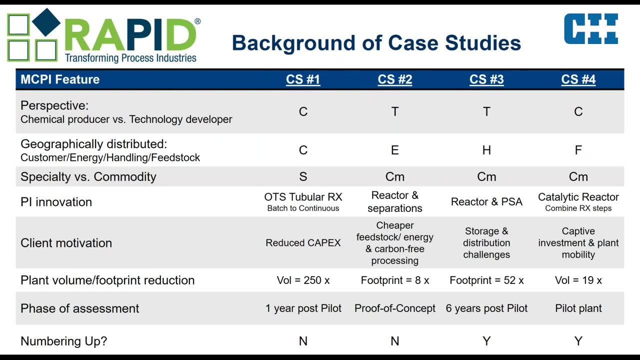 brownfield and that and that this little plant, this specialty chemical plant, usually sits in a larger in the context of a larger plant, so that that you know usually sits in a larger in the context of a larger plant, so that that you know qualifies it as brownfield. the same is true of 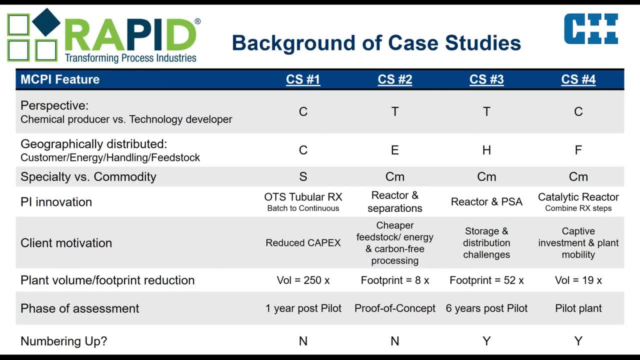 qualifies it as brownfield. the same is true of number four and I think number number three. number four and I think number number three can vary either way. number two mostly can vary either way. number two mostly greenfield. okay, I have another question. can you share more about the emergency case study that was studied? 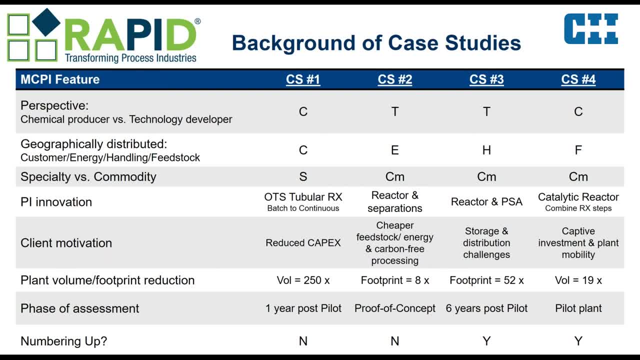 emergency case study? yeah, what would is the reference to now? that's yeah, that's all I show there in the question. can you share more about the emergency case study? emergency, nope, Nope, Nope, Yeah, I don't think any of our case studies fit into the emergency. 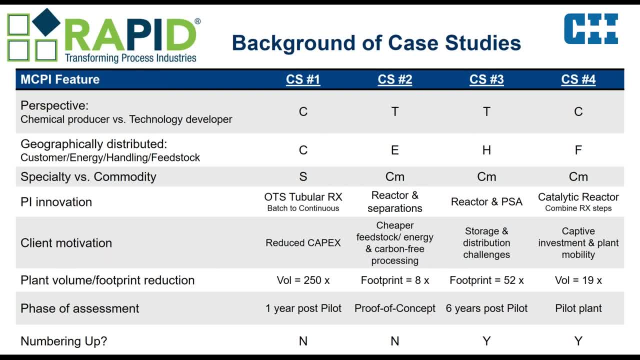 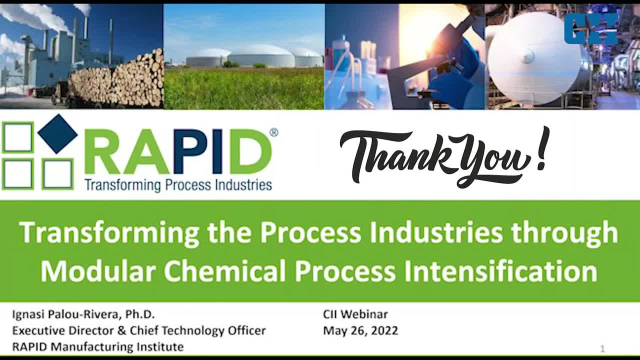 Okay, Well, the question came from Jason. So, Jason, if you're still out there, feel free to follow up with Jim directly on the email address that was shared. Otherwise, everyone. that was the last question I had. I had some positive feedback from some of the attendees today. They said thank you for all the great examples. 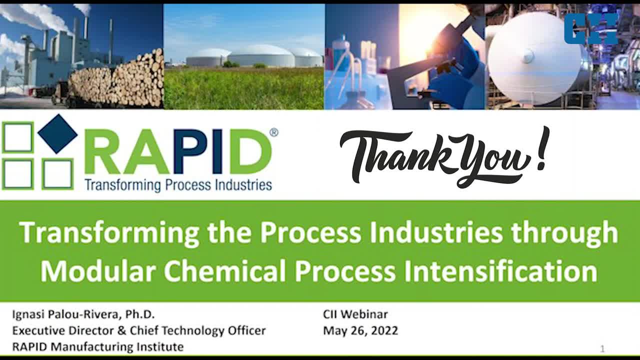 Thank you all for your time. We appreciate your attendance today. Again, feel free to reach out to our team if you have any follow up questions. We are more than happy to circle back with you after the fact. So thank you to our presenters today: Ignacy Olivier and Jim.